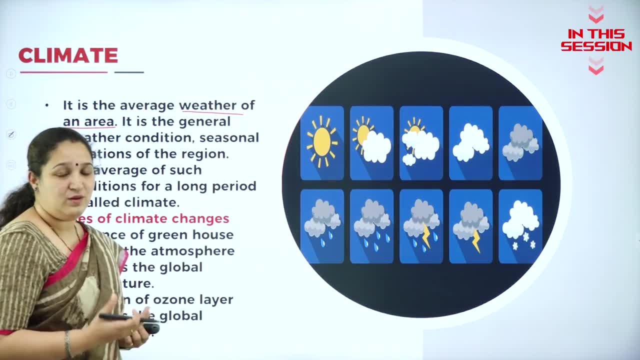 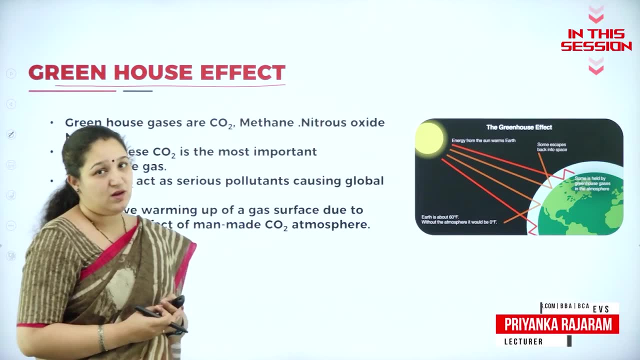 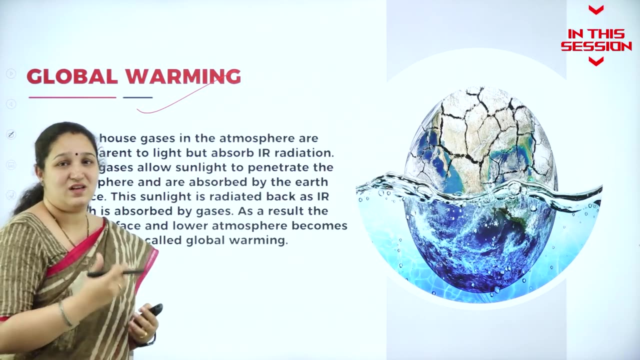 So what is the weather of a particular area? We call that as the climate. This is one of the causes for the climate change. So what exactly is greenhouse effect? Because of greenhouse effect, the entire earth's surface temperature has increased. Stop deforestation and start afforestation. 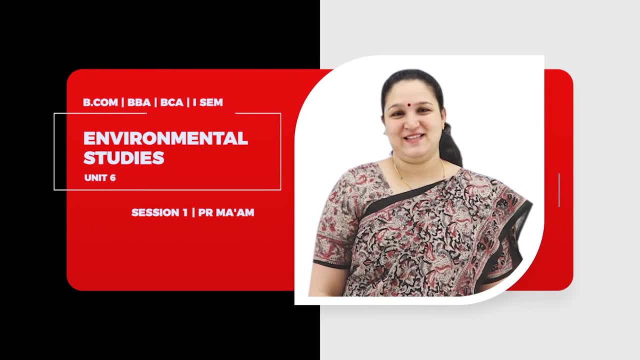 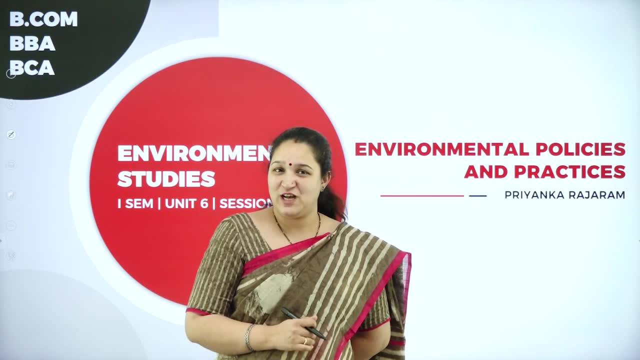 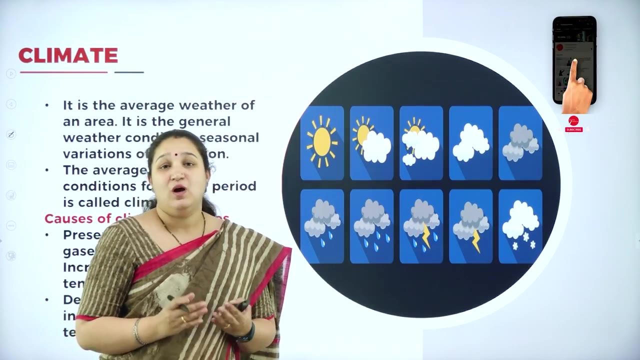 Hello, my dear students, Welcome back. Today I'm going to start with a new chapter: environmental policies and practices. Before I go into the detail about this chapter, we are going to learn what are the effects or what are the damages which we have done to the 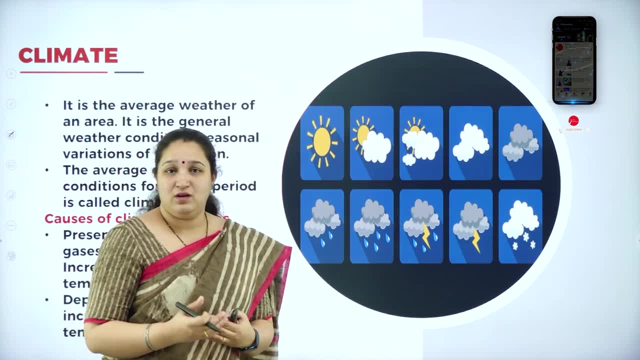 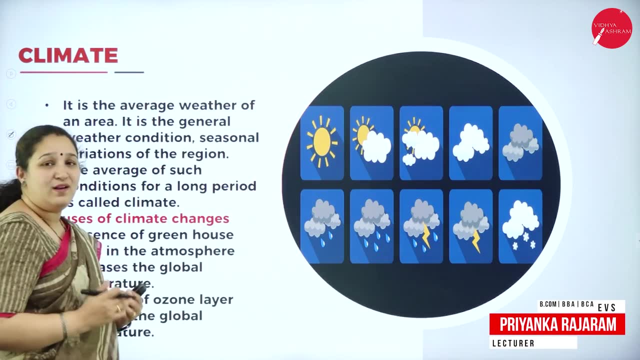 environment and what are the policies? which has been passed, or which is the act or a law which is passed or which is not passed? So let's get started. Let's get started So that we can protect our environment. What is climate? Climate is the seasonal variation. 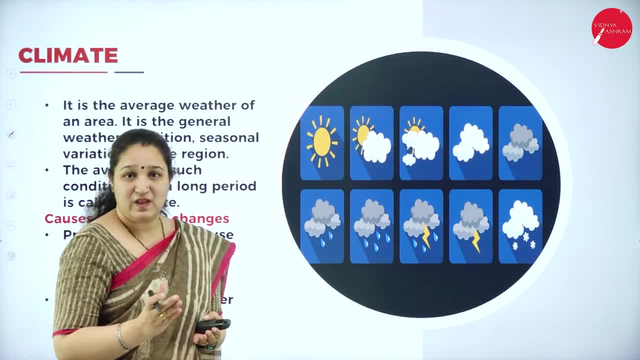 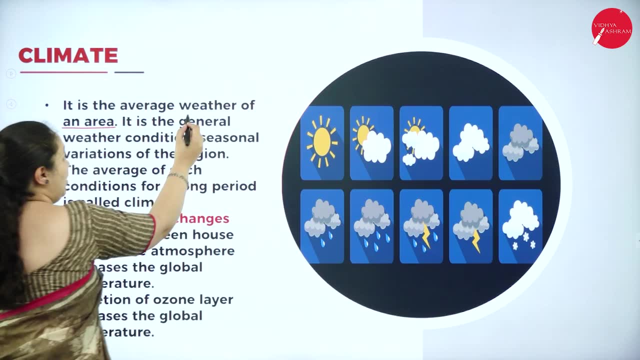 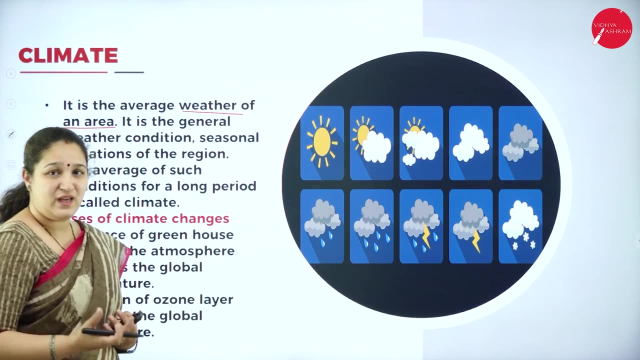 or a weather in a particular region. Am I right? What is climate? It is the average weather of an area. What weather? How is the weather? Whether the temperature is high or low, whether it's cold, whether it's very hot, or you know whether humidity is. 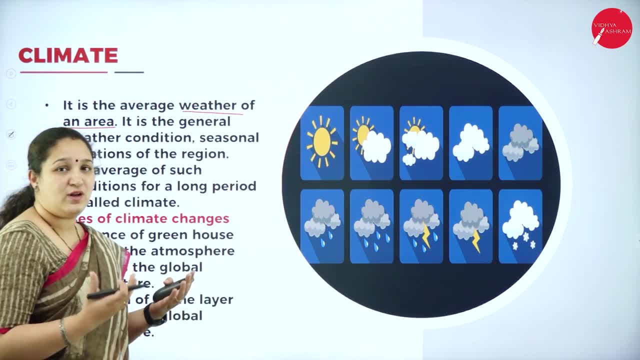 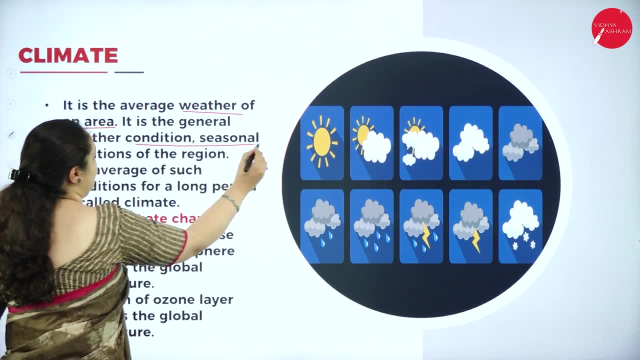 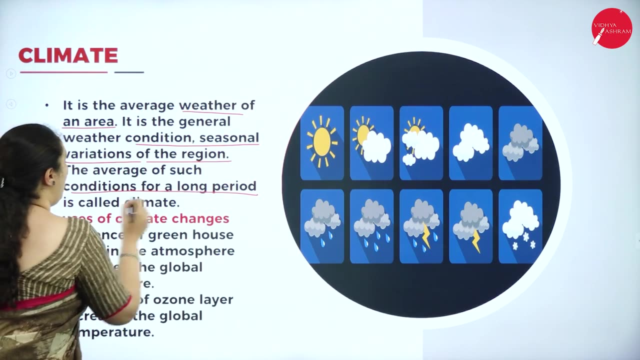 high. So what is the weather of a particular area? We call that as the climate. So it is general weather condition, seasonal variations of a particular region And the average of such conditions for a long period is called as climate. So what is the condition which is there? 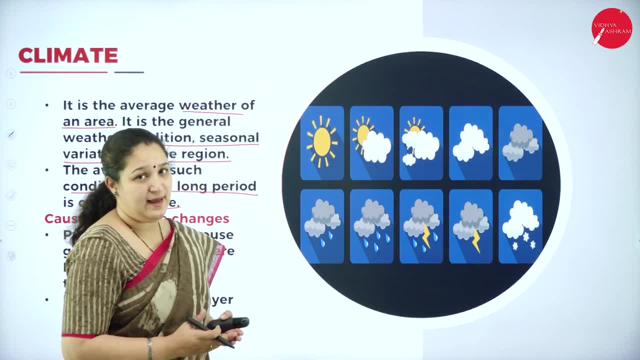 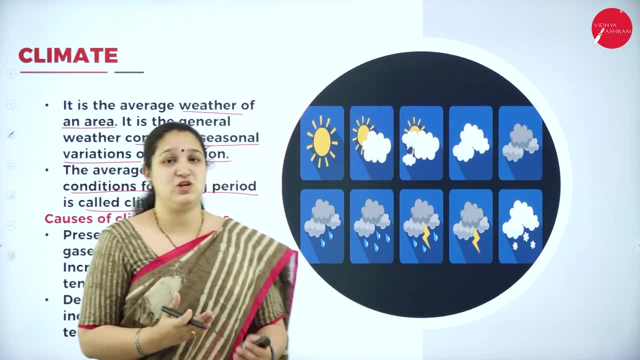 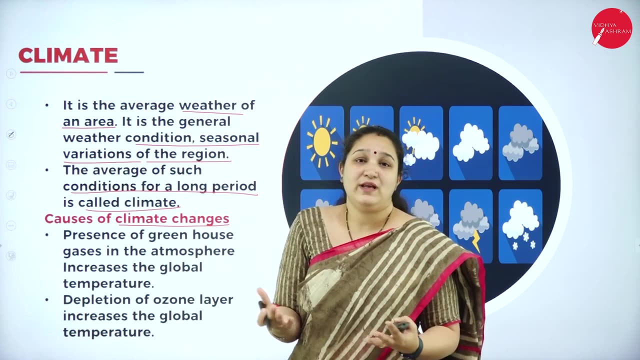 For a very long period. if you see, then we call it as the climate Okay, So causes for climate change. Nowadays, if you see, there is a lot of climatic changes which is happening. It will rain when it is not supposed to rain. It is too very hot or, you know, it is too very cold. 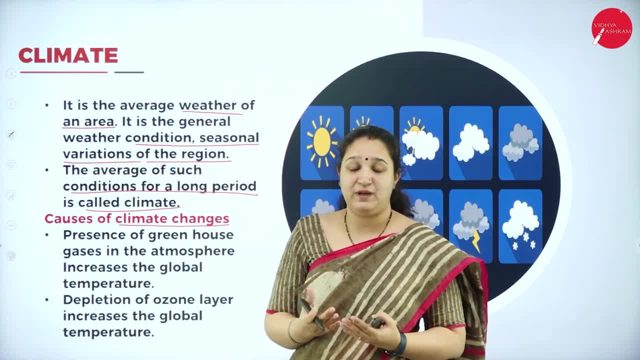 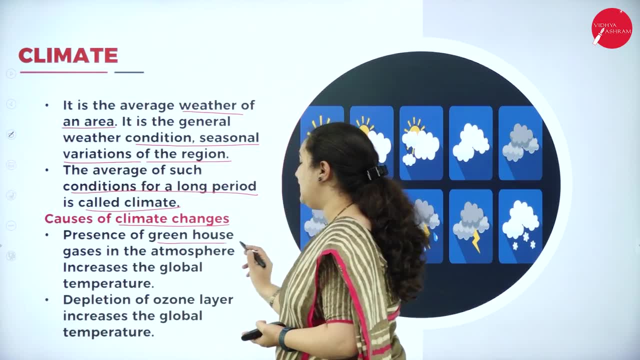 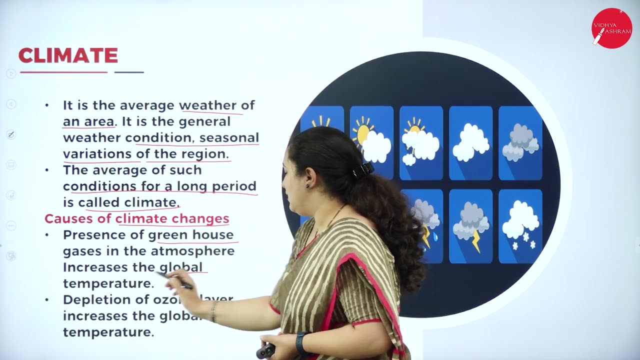 during winter. So there are many changes which is happening And what are the main causes for climate change? That is, presence of greenhouse gases is the main cause of climatic change And also due to greenhouse gases, there is a lot of climate change. So there are many changes. 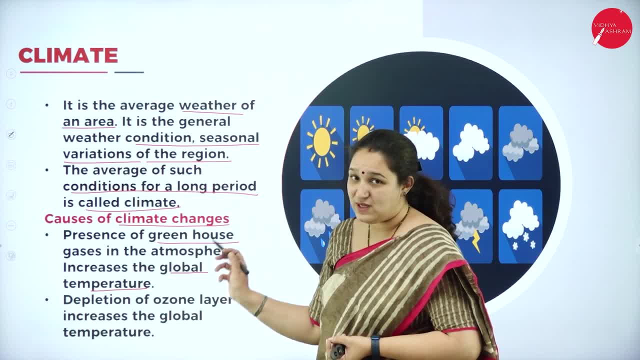 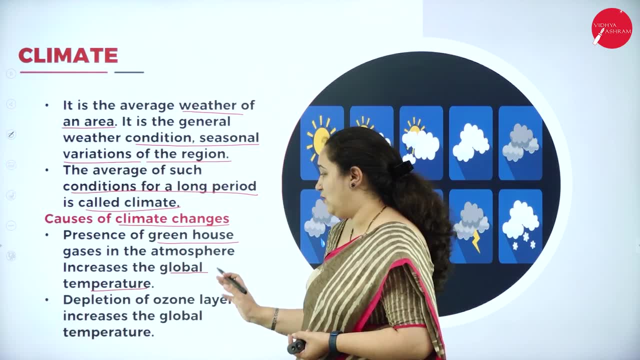 which are happening. There are a lot of greenhouse gases. There is global temperature increase, which we call it as global warming. More further when we go, I will explain about what are greenhouse gases. what is the meaning of global warming as well. Okay, And depletion of ozone layer. 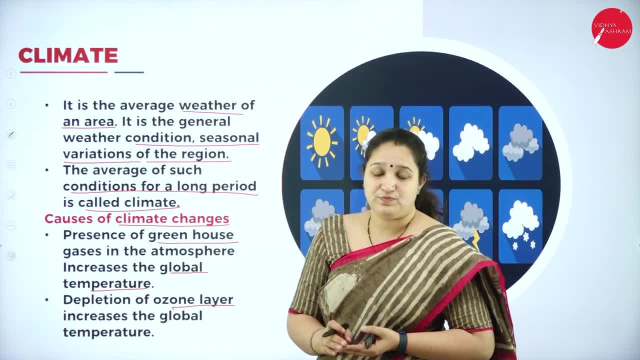 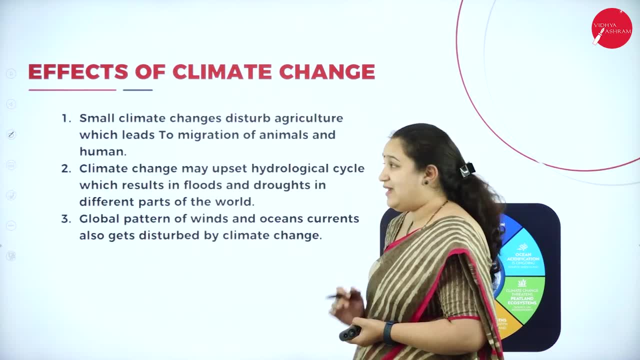 is another cause for climatic change. So what are the effects of climate change? We can see that small climate change disturb the agriculture, which leads to migration, migration and the like. So what are the effects of climate change? So what are the effects of climate change? 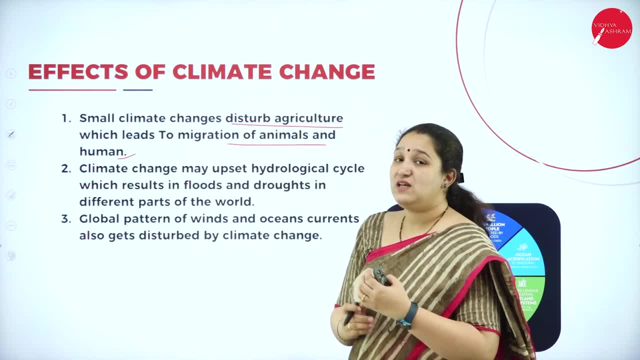 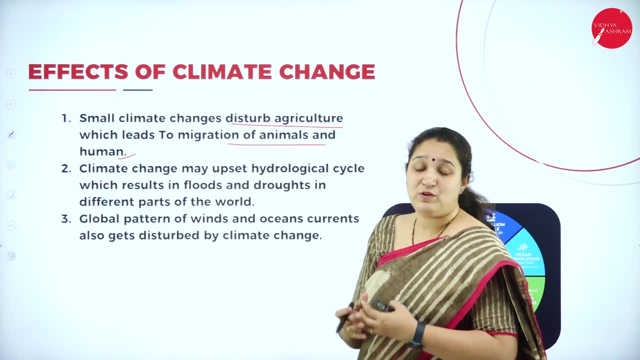 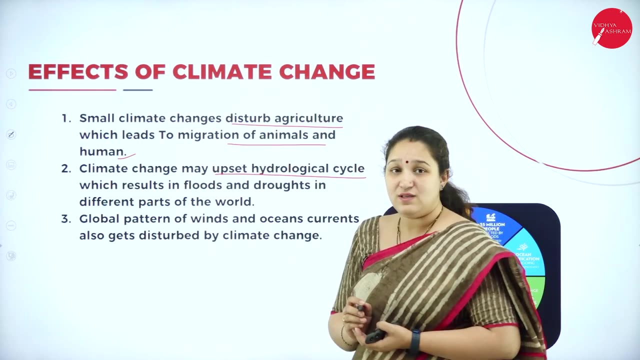 of animals as well as the humans. so there is pattern of agriculture will completely change, due to which, you know, there can be migration of people from one place to another, just because there is a climatic change. also, climate change may upset the hydrological cycle, that is, the water. 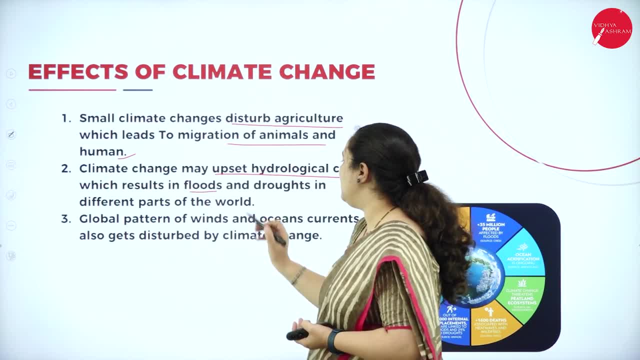 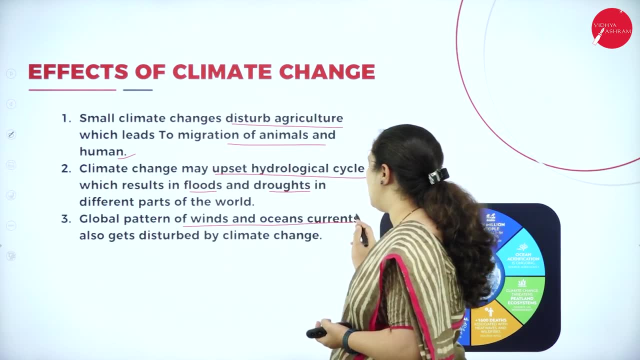 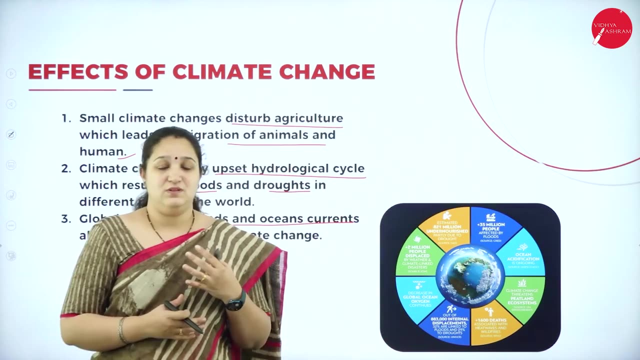 cycle can be completely upset and it might result in flood or in drought in different parts of the world, as also global pattern of winds and ocean currents also get disturbed due to the climatic change. so when the climate changes, you know the agricultural crop, there is a lot of loss for. 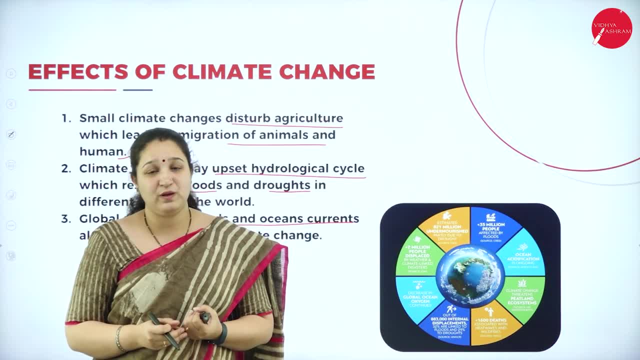 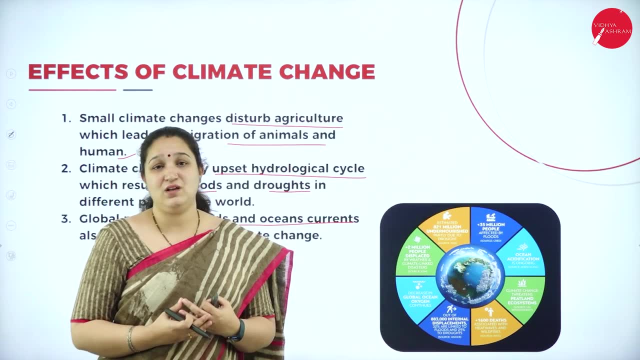 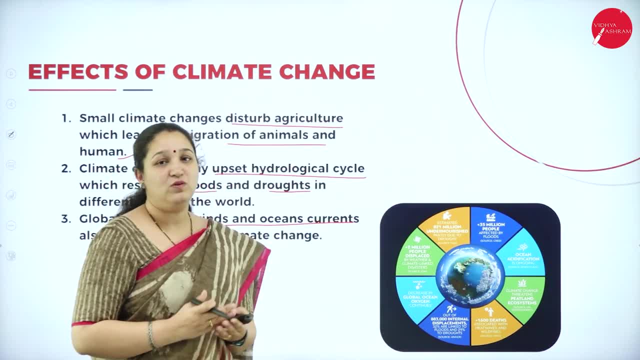 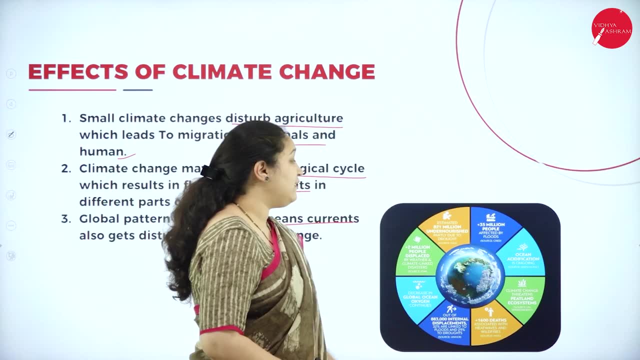 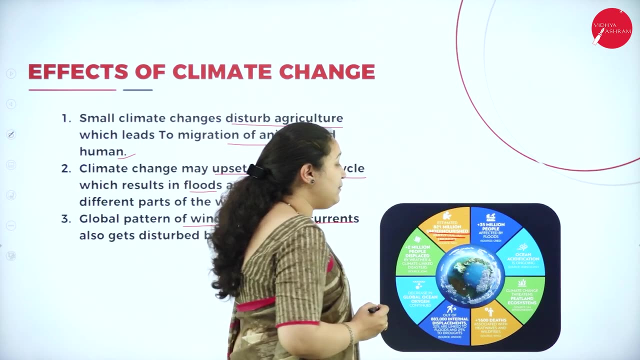 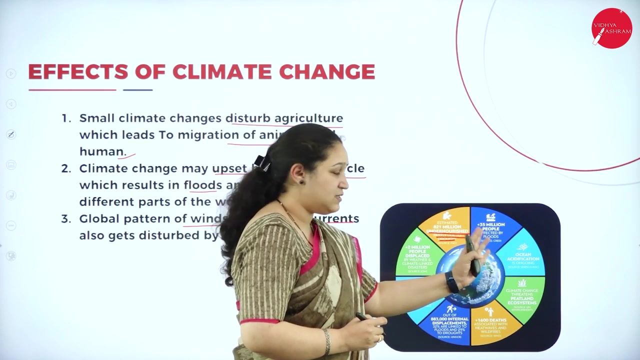 changes, which is happening because of, you know, climate change. so you can see that there is estimate of 821 million undernourished due to the drought. okay, 35 million people affected by flood. ocean acidification is continuously going on process and also climate change threatens peat. 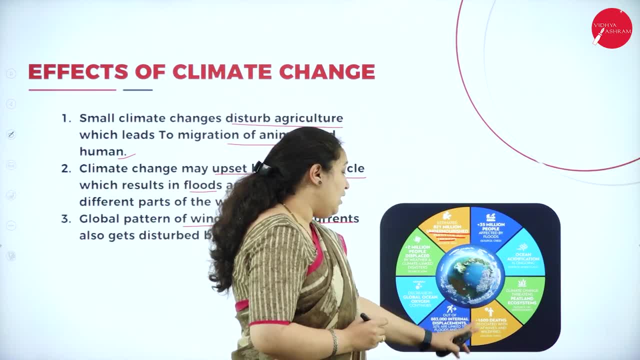 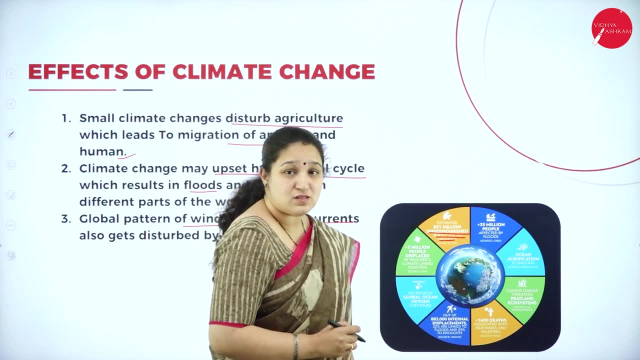 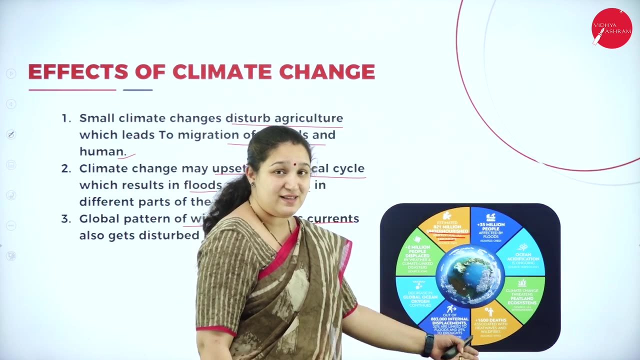 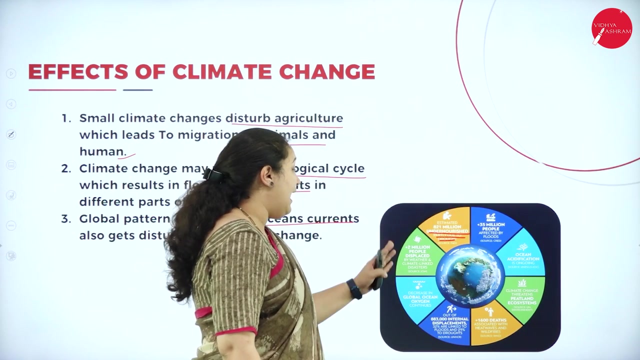 land ecosystem. that is again 1600 deaths- is associated with the heat waves and the wild fires. okay, that is the fire in the forest, or there is so much heat that it is led to 1600 deaths all over the world, and it is also having, you know, decrease in global ocean oxygen continues as well as two million people are. 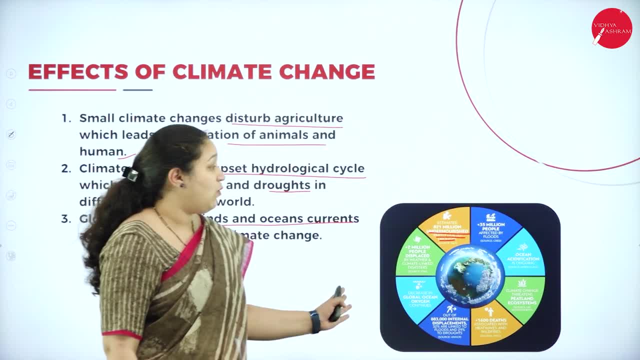 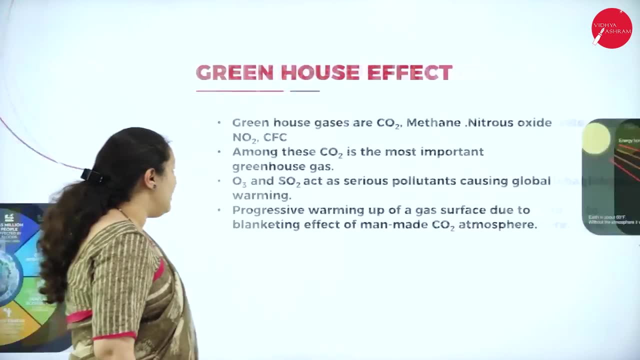 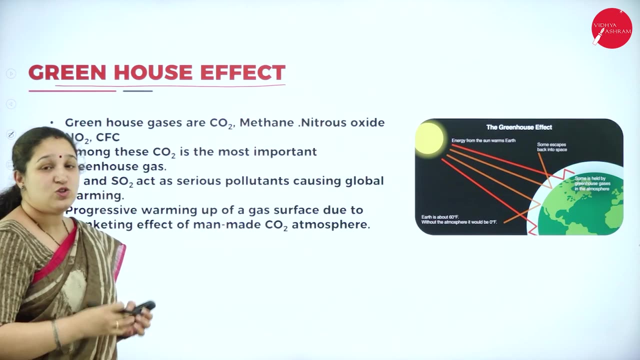 displaced by the weather and the climate change. so you can see what are the effects which we have around the world, you know, due to the climate change also. next is: what is a greenhouse effect? this is one of the causes for the climate change. so what exactly is greenhouse effect? now, what happens is: 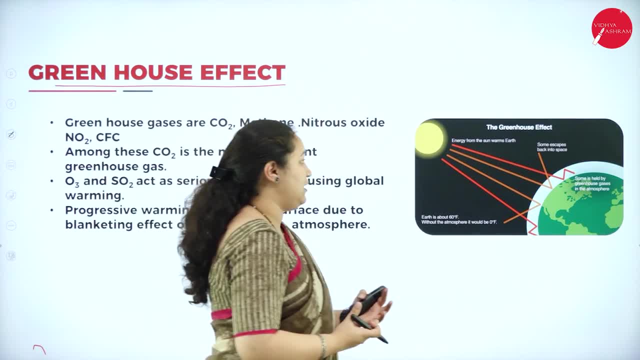 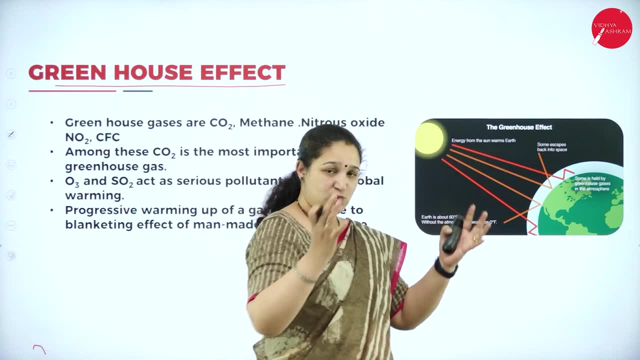 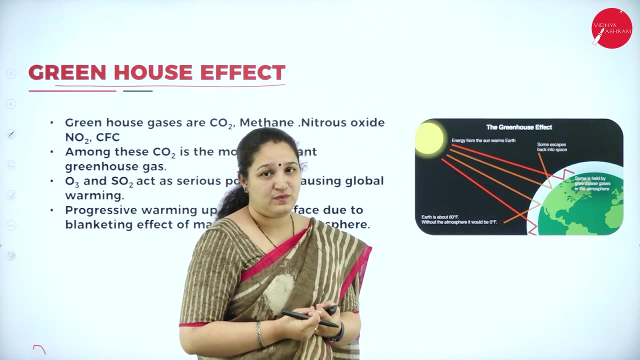 from the sun, whatever sunlight or the energy. what is there? energy from the sun falls on the earth surface and around the earth surface we have atmosphere in which there are gases which will absorb these radiations from the sun. okay, and because these, you know, gases or the in the 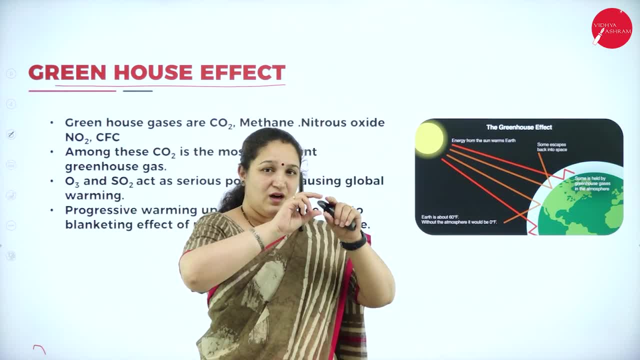 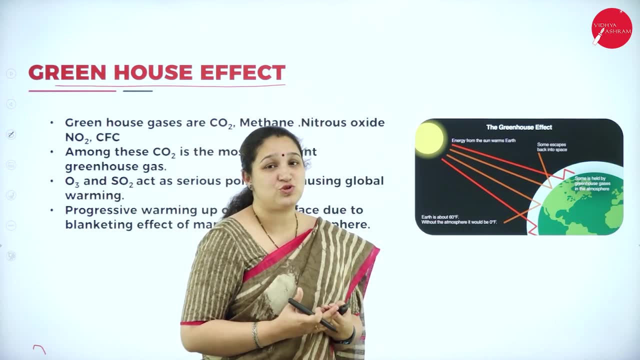 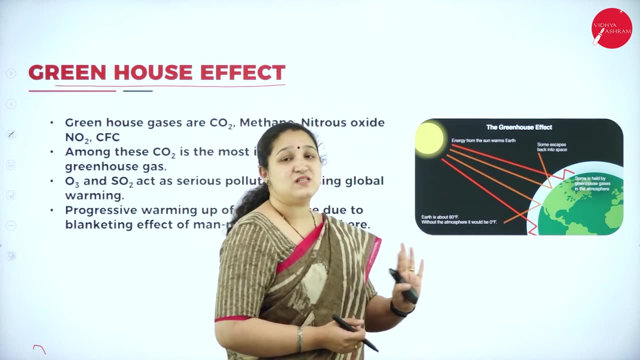 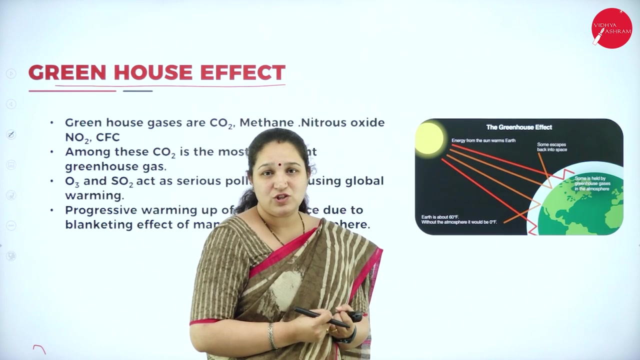 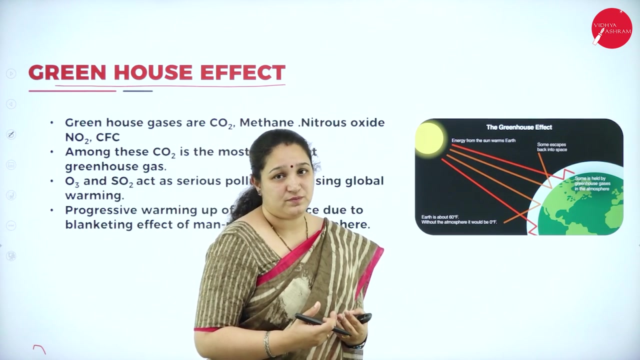 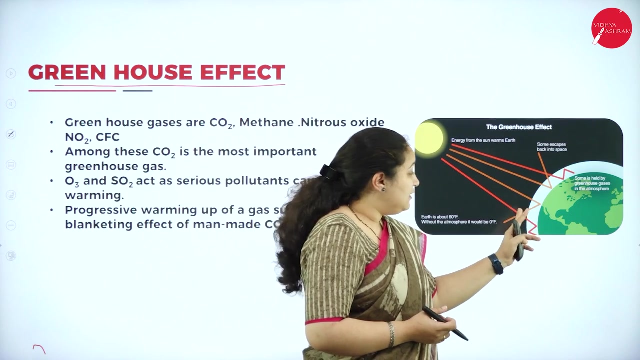 atmosphere, there is absorption of radiation. there is a region around the earth which is warm and makes us a comfortable place to live. okay, earth is about 60 degree fahrenheit temperature. without the atmosphere, it would be just zero degree fahrenheit. okay, only because there is atmospheric gases which can absorb the energy from sun and, you know, can warm up the entire surface of the earth. we can live on earth. okay. now what is greenhouse effect, if you ask me? as the pollution is increasing, the gases in the atmosphere is also increasing, that is, gases like carbon dioxide and methane, which is having the high capacity to absorb this radiation. 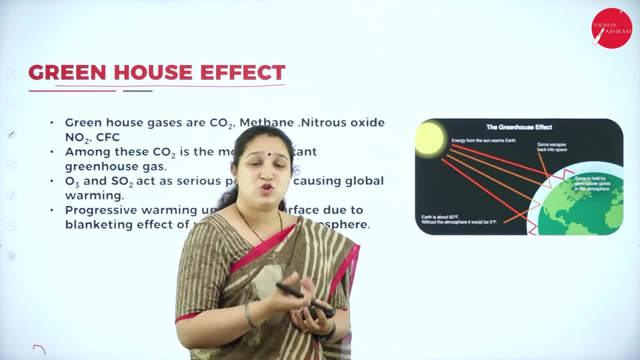 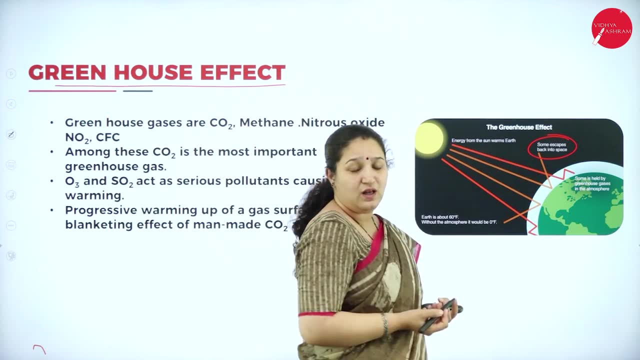 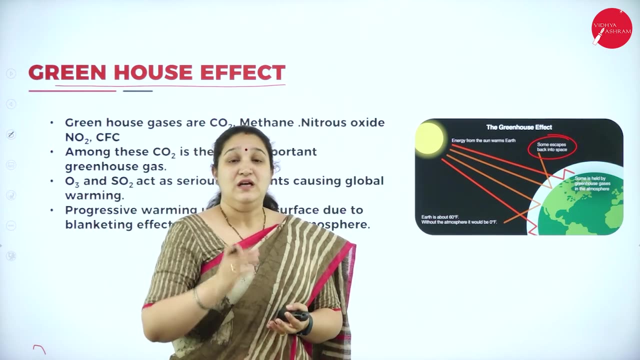 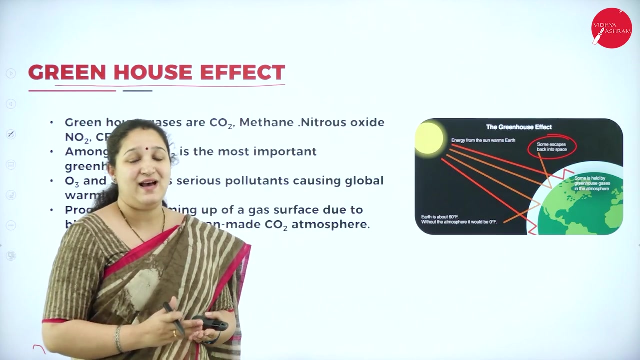 which is having the high capacity to absorb this radiation, radiation, well, The extra radiation, some radiations, you know it can escape back into the space as well. But because the amount of greenhouse gases is increasing in the atmosphere, the earth's surface temperature is increasing And this effect is called as greenhouse effect. 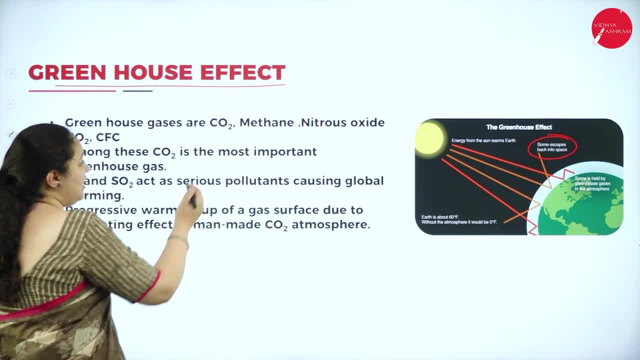 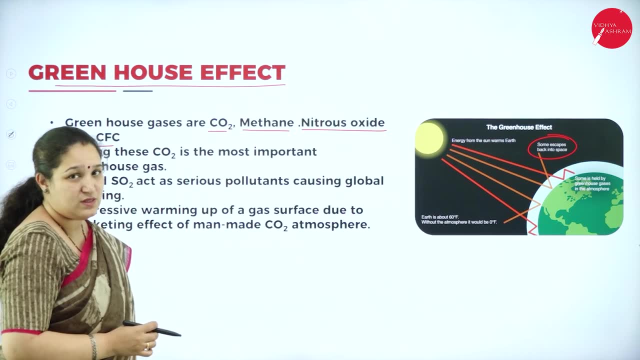 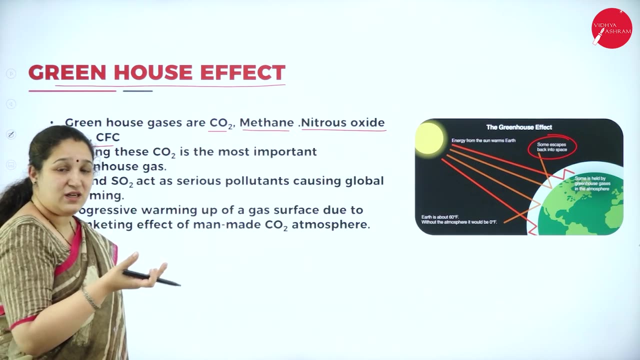 Okay, So what is it? Greenhouse gases are carbon dioxide, methane, nitrous oxide, nitrogen dioxide, CFCs, that is, chlorofluorocarbons. Okay, All these are considered as greenhouse gases which can have or which has the capacity to absorb the energy of the sun. 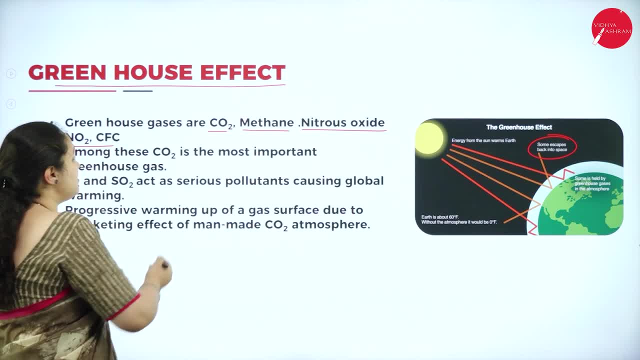 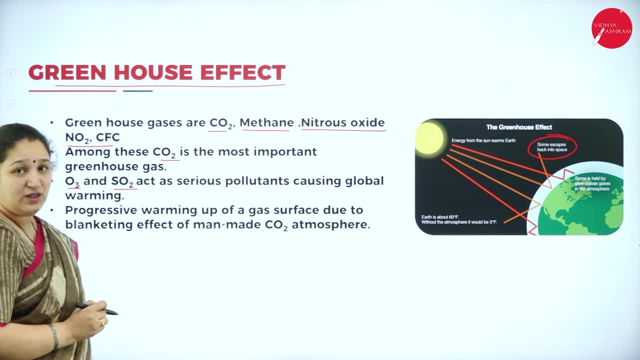 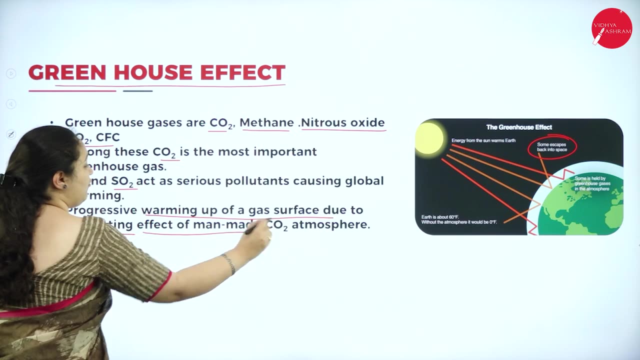 very well, Okay. Among these, carbon dioxide is the most important greenhouse gas. Also, ozone and SO2 act as serious pollutant, causing global warming and progressive warming up of the gas surface due to blackout. So the blanketting effect of man-made carbon dioxide in the atmosphere is called as greenhouse. 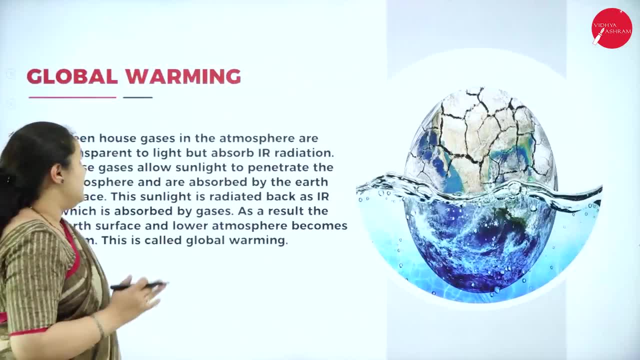 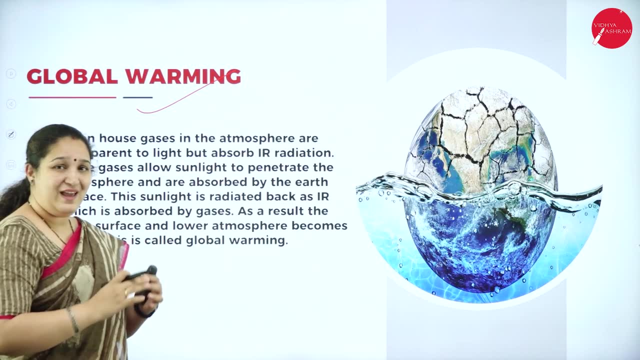 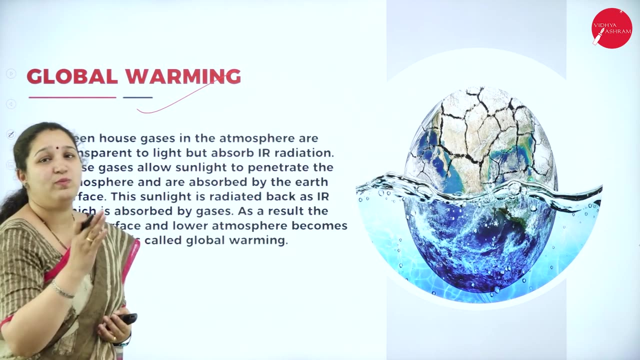 effect. Okay, Now. next is about global warming. Now, what is global warming? Because of greenhouse effect, the entire earth's surface temperature has increased, And this is called as global warming. Okay, So what is it? Greenhouse gases in the atmosphere are. 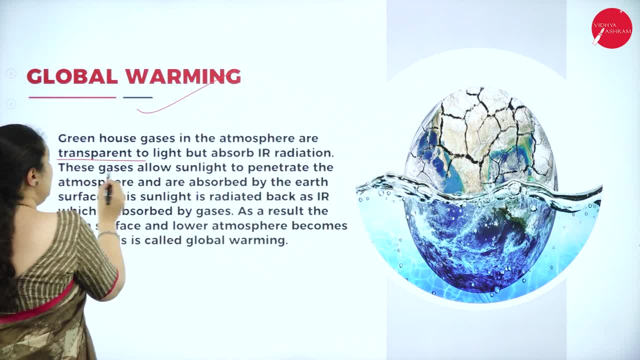 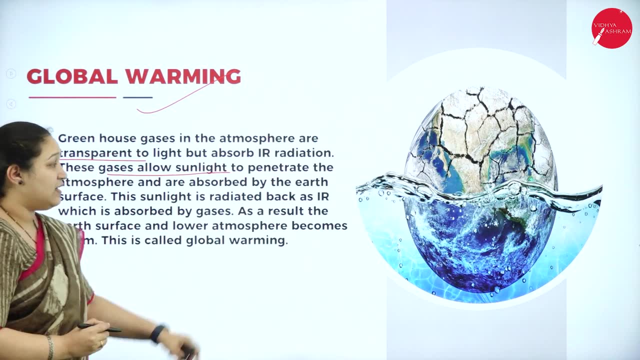 transparent to light but absorb radiation. These gases allow sunlight to penetrate the atmosphere and are absorbed by the earth's surface. This sunlight is radiated back as IR, that is, radiation- infrared radiation- which is absorbed by the gases. As the result, earth's 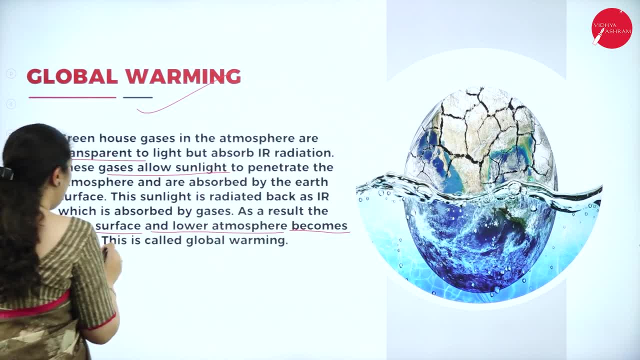 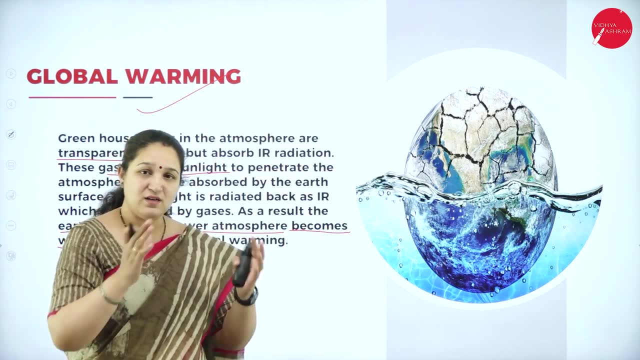 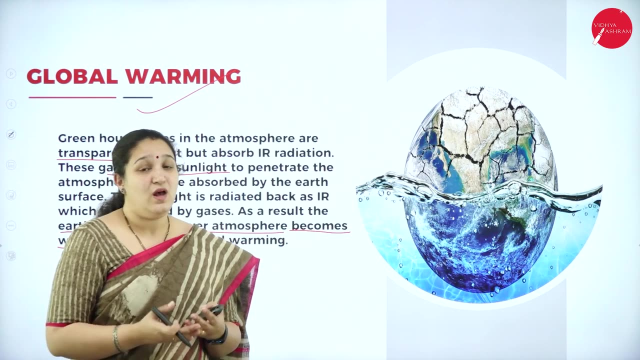 surface and the lower atmosphere become warm, And this is called as global warming. That is due to the greenhouse effect. The entire surface of the earth's temperature is increasing by 2, or 3 degree Celcius, or even more, and this is called as global warming. Now, what is the effect of global warming? If you see the 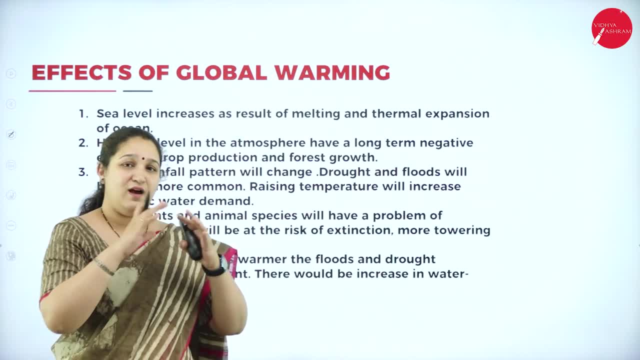 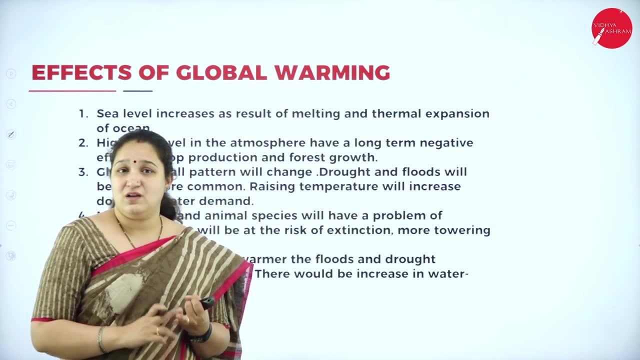 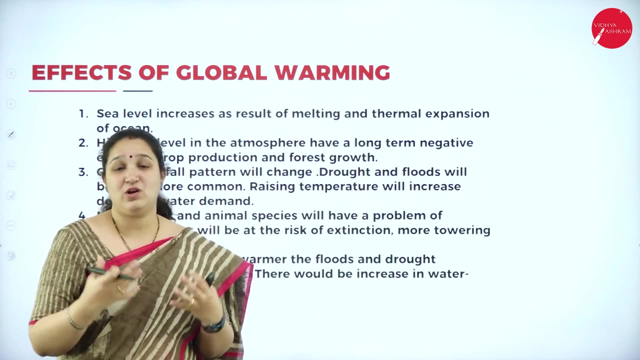 effects of global warming. one thing is: because the entire earth's surface temperature has increased, the glaciers can start melting. The plants, you know, cannot live in very high temperature. there might be animals which cannot, you know, take up or can live in that particular temperature. 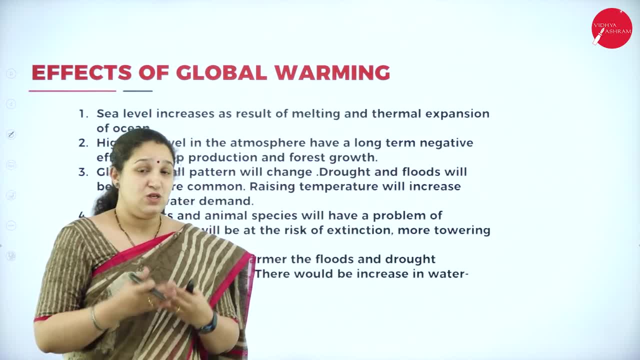 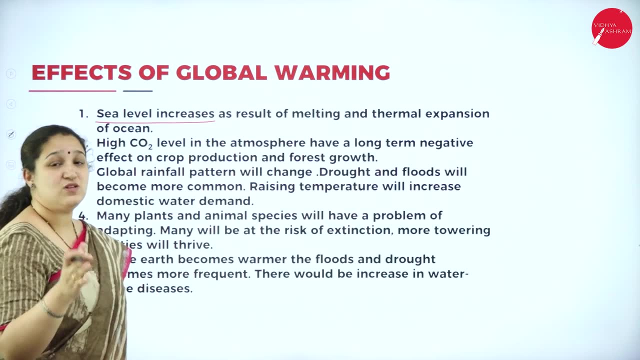 or a higher temperature, all such problems will start. so we'll see what are the effects in detail. sea level increases. how is the sea level increasing? that is because of the melting and the thermal expansion of the ocean will take place. melting of the ice, okay, and or the glaciers. 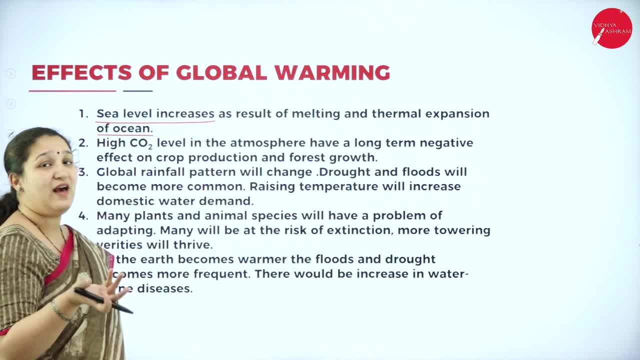 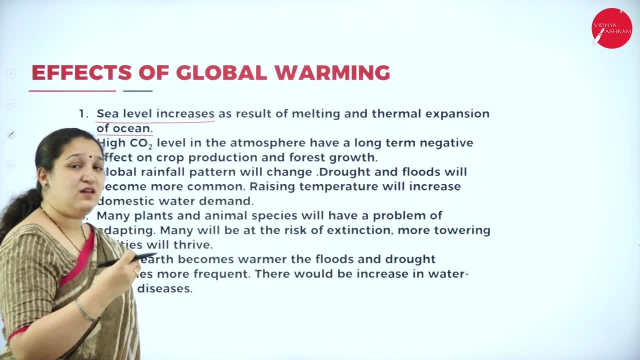 and because of which what? there is expansion of the ocean. already we have 79 percent of ocean or sea in the world and very small amount of land is there and still the ocean content is increasing. that means land content is decreasing. there is submergence, you know the coastal areas can get. 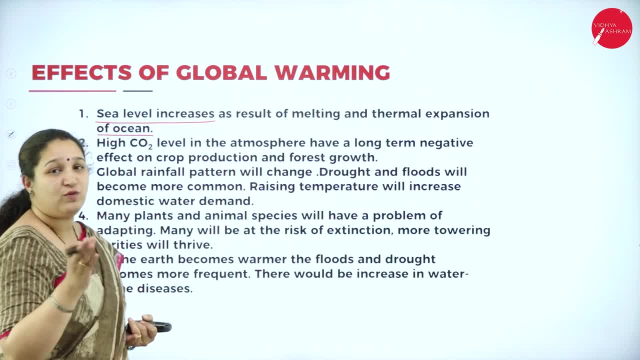 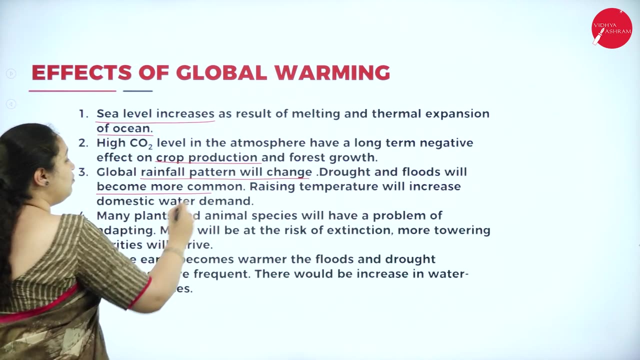 submerged in water as well. okay, that is one of the major effects of global warming. next is high carbon dioxide level in the atmosphere have a long-term negative effect on crop production and forest growth. global global warming. rainfall pattern will change, okay. drought and floods will become more common, raising temperature. 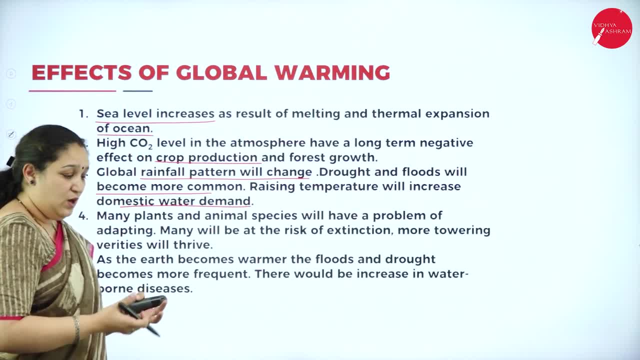 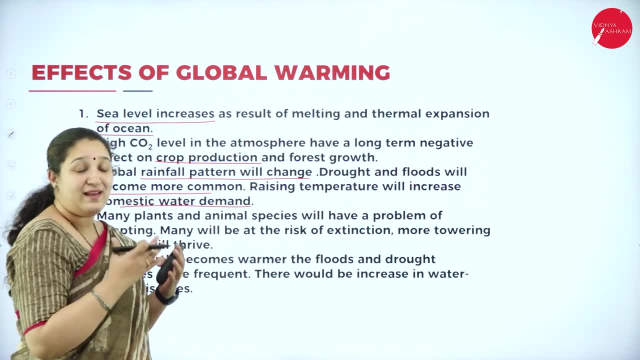 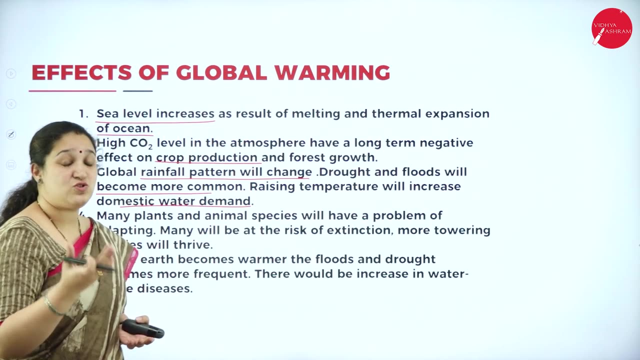 will increase the domestic water demand because there will be water evaporation will take place very easily, due to which the water cycle also will be disturbed, okay, and there will be scarcity of water. it will start raining when it's not supposed to rain and, you know, the floods can also increase. 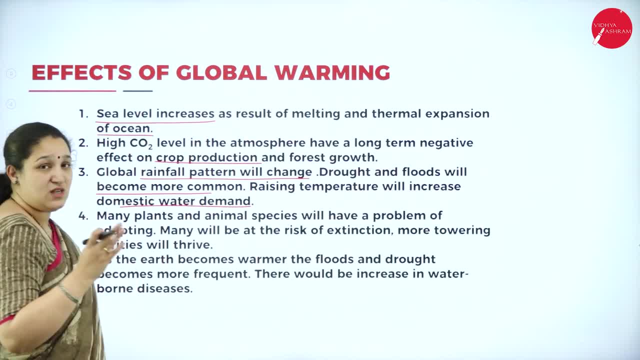 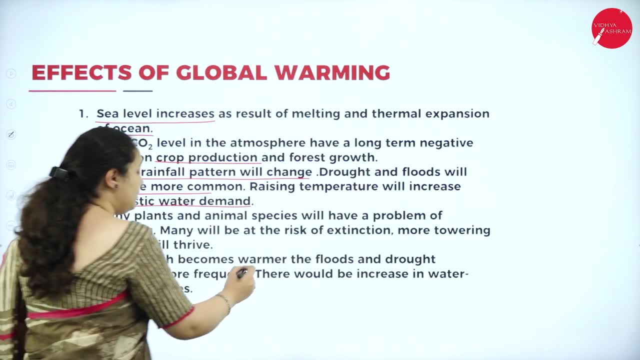 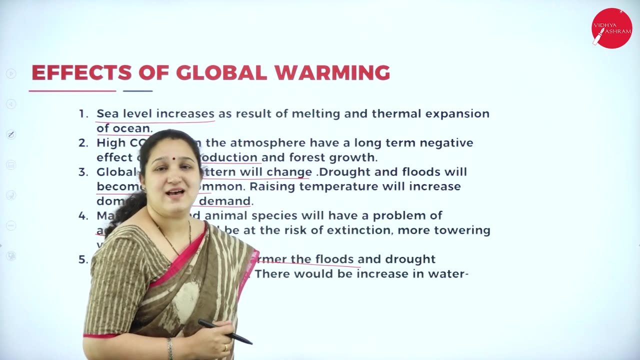 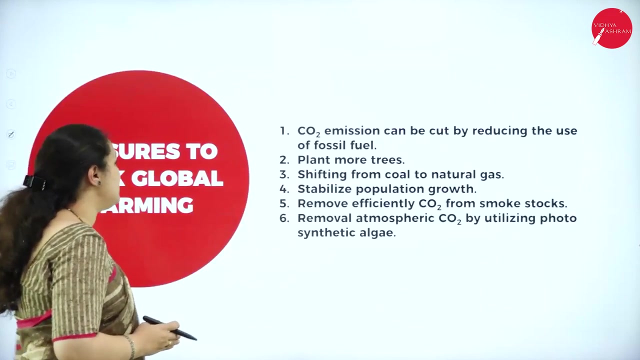 drought also can increase. many plants and animal species will have a problem for adapting. many will be at the risk of extinction. as the earth becomes warmer, the floods and the drought becomes more frequent, and this would increase the waterborne diseases as well. so these are some of the major effects of global warming we can see. okay. next is about the measures to 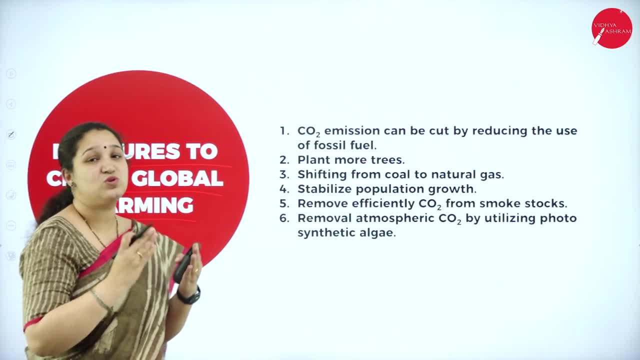 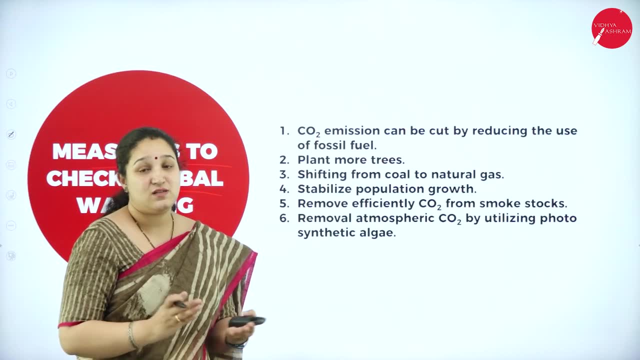 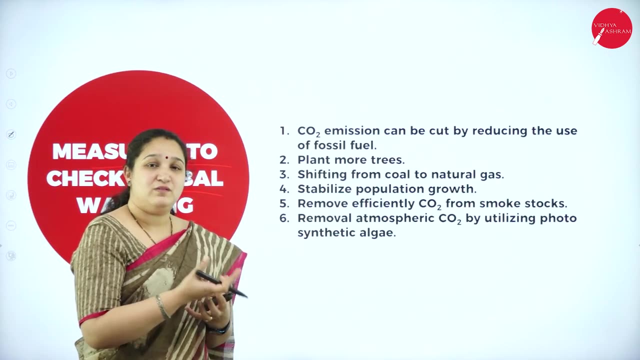 check global warming. how is that we can reduce global warming? first thing, what we need to do is stop deforestation and start afforestation. that is, we need to plant more trees, because trees will take up the pollutants you know. it can take up toxic chemicals, it can take up carbon dioxide and 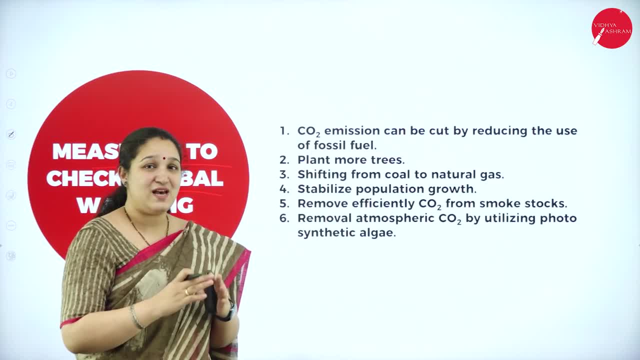 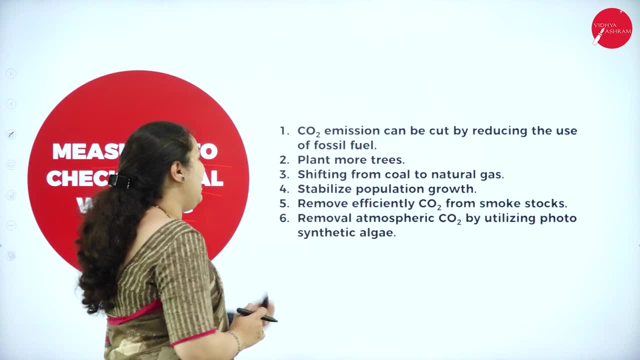 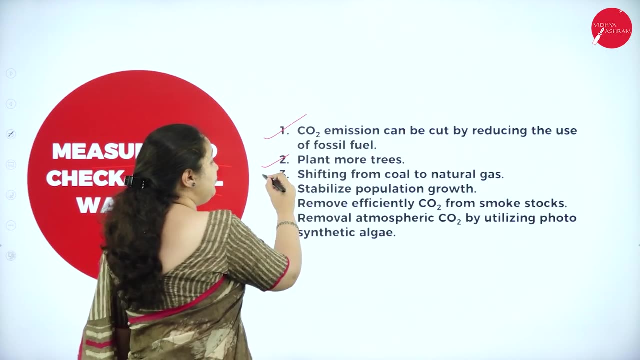 get it converted to oxygen. so once these greenhouse gases content will be reduced, then global warming can be immediately tackled, isn't it so? plant more trees. carbon dioxide emission can be cut off by the use of fossil fuels, shifting from coal to natural gas. use of coal should be reduced. 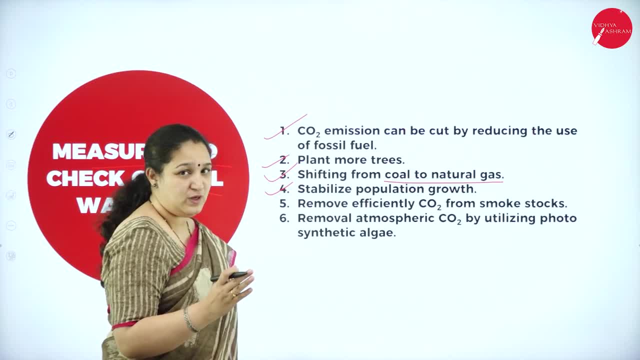 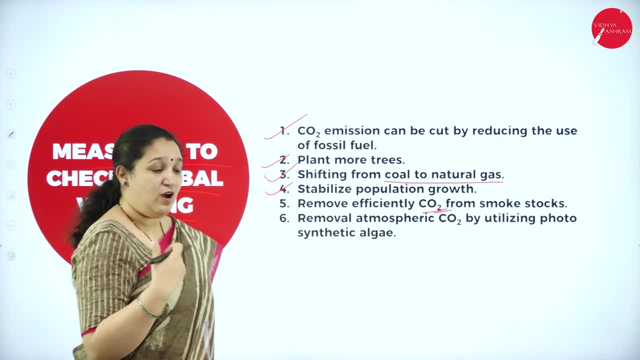 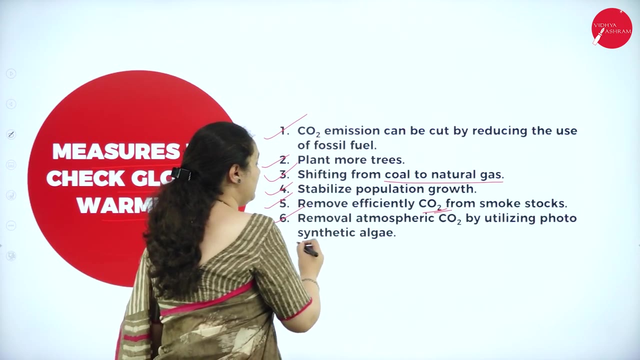 stabilize population growth. we have to check on the population growth. remove efficiently carbon dioxide from smoke stocks, that is, from the industries. you have to check on the carbon dioxide gas which is getting released. removal of atmospheric carbon dioxide by utilizing photosynthetic algae. that is more and more photosynthetic algae. if it is grown, it will. 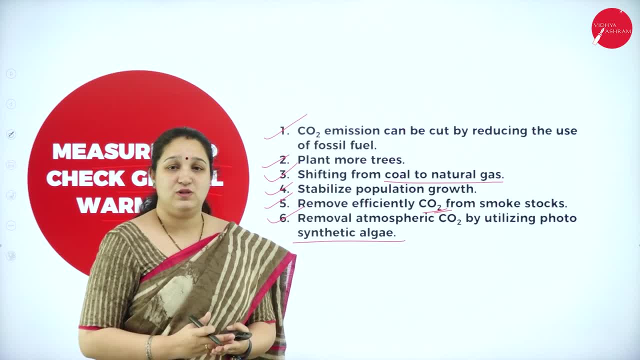 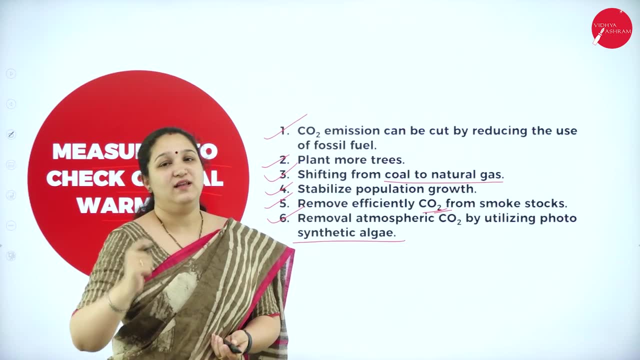 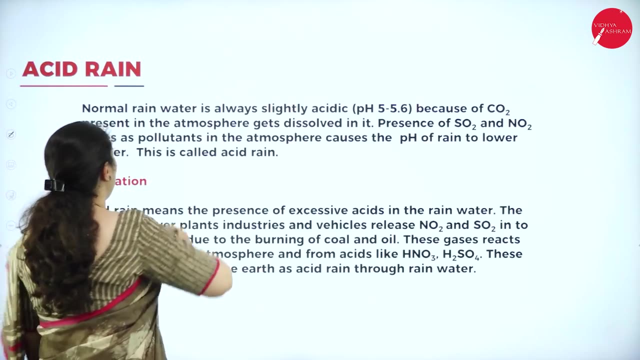 take up the carbon dioxide and get it converted to oxygen and, due to this, carbon dioxide content can be tackled, and this will directly tackle what the greenhouse effect and the global warming. so that's about the measures which we can take. next is about acid rain: acid rain. i have already 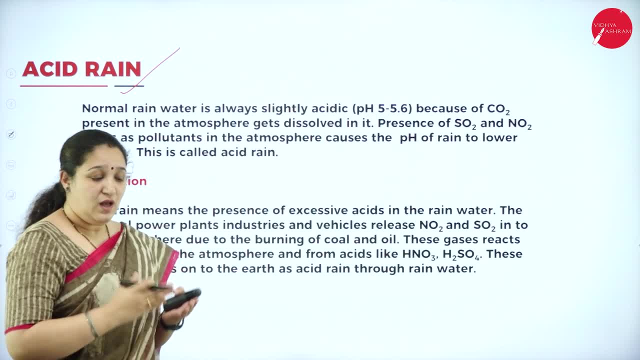 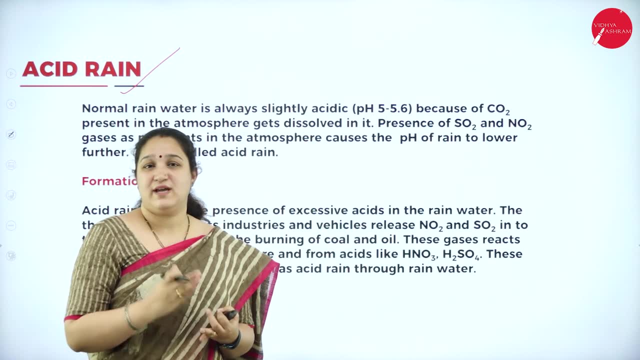 explained once, but once again i shall explain what is it in the atmosphere. we have lot of carbon dioxide, nitrous oxide, like nitric oxide, and you know it is nitrogen dioxide, different oxides of nitrogen. we have different oxides of sulfur. we have like sulfur dioxide, sulfur dioxide, etc. these are all air. 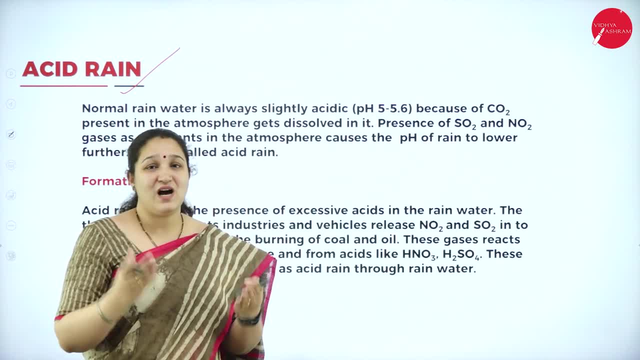 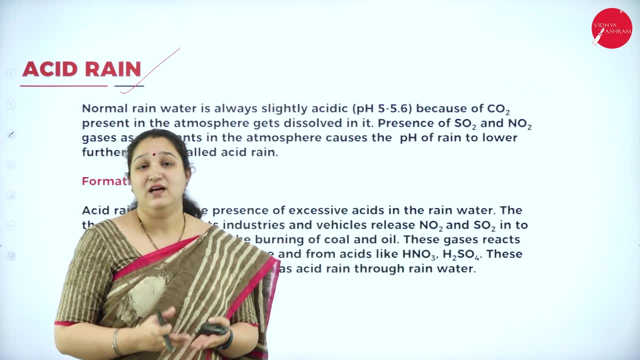 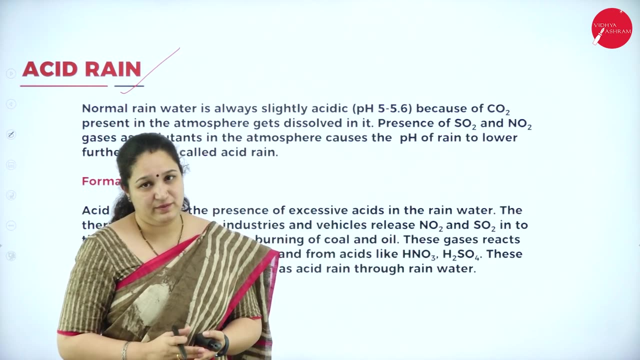 pollutants which is there in the atmosphere. now, when it starts raining, okay, the water will combine with these gases to produce acid and the rain which comes down will be acidic in nature and this is called as acid rain. okay, so what is it? the normal rain water is always slightly acidic. that is five to five. 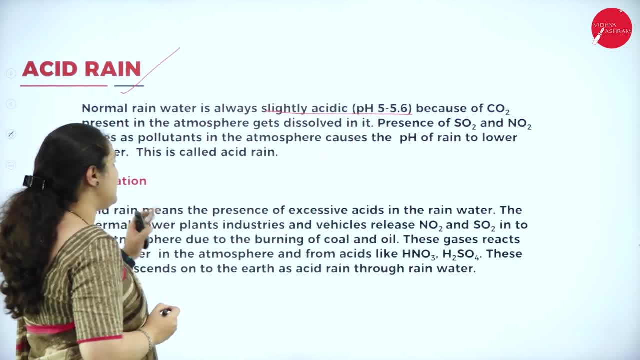 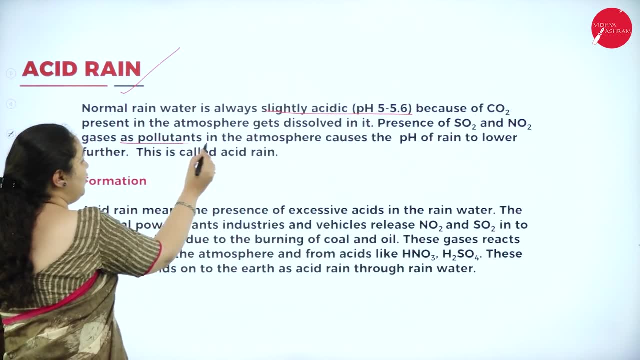 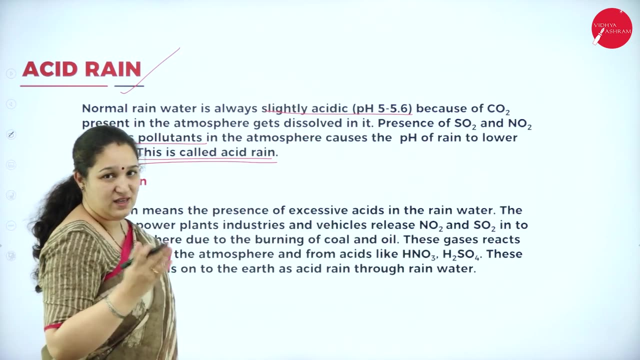 point six: ph because of carbon dioxide present in the atmosphere gets dissolved in it. presence of sulfur dioxide and nitrogen dioxide gases as pollutants in the atmosphere causes ph of the rain to lower further and this is called as acid rain. as i've explained, what or how is acid rain formed? okay, acid rain is formed in closed water. we asked this question, ok. 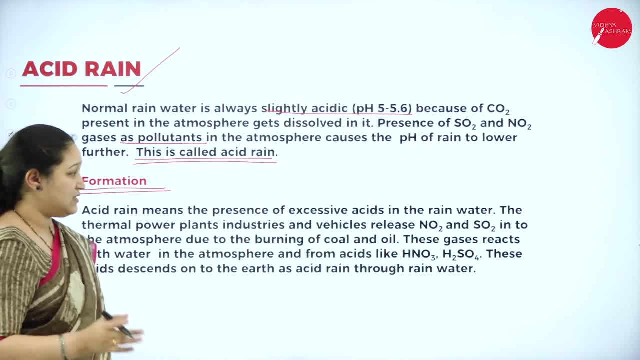 right acid rain how this acid rainishops formed in the rain water dezeasers many electric molecule. there was a number of different libraries in our inать atat, pastorytica today called as acid rain here by by load acid sein toי. it means presence of excessive acid. as I told you, the thermal power plants and industries vehicle. 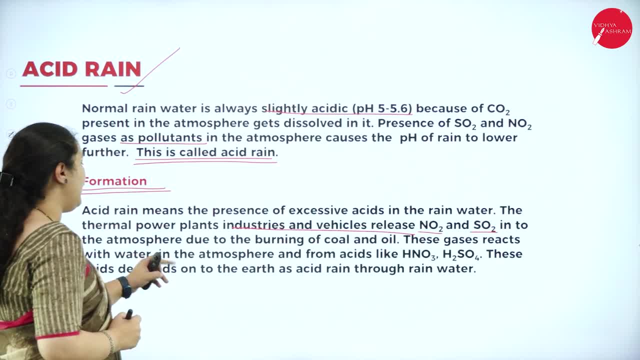 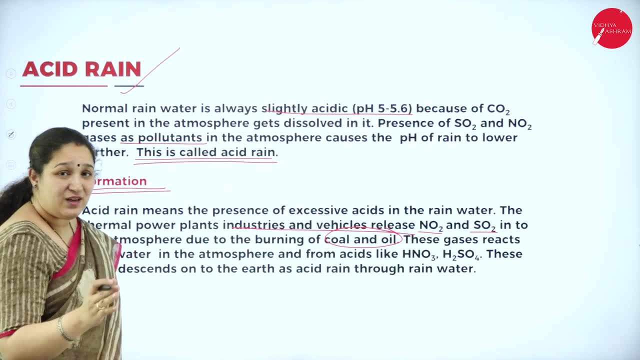 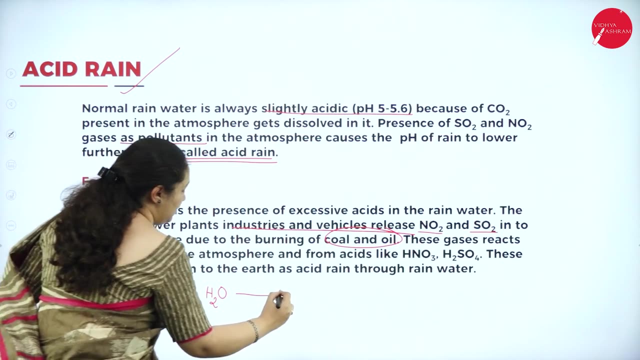 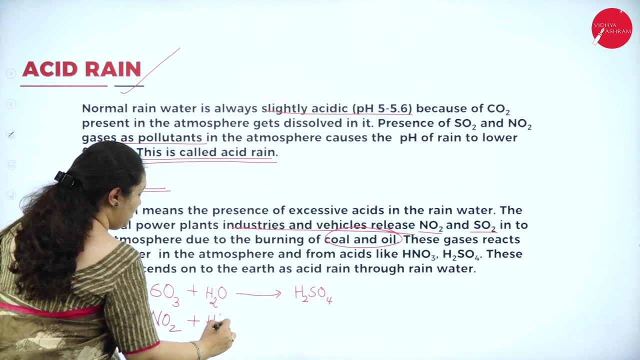 release nitrogen dioxide and sulfur dioxide gas into the atmosphere due to burning of coal and oil, and these gases react with water. I can also write the reaction for y'all. for example, SO3- I have- reacts with water to form. H2SO4 and NO2, if I have, it reacts with water to form. 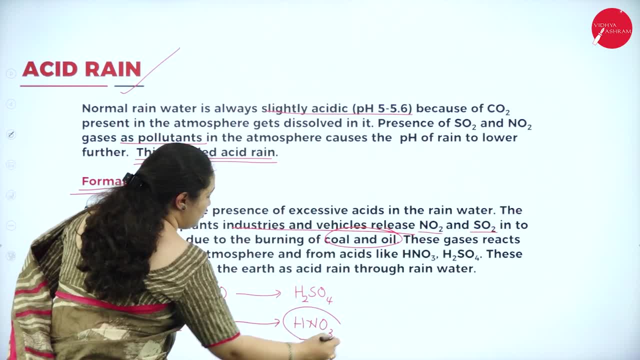 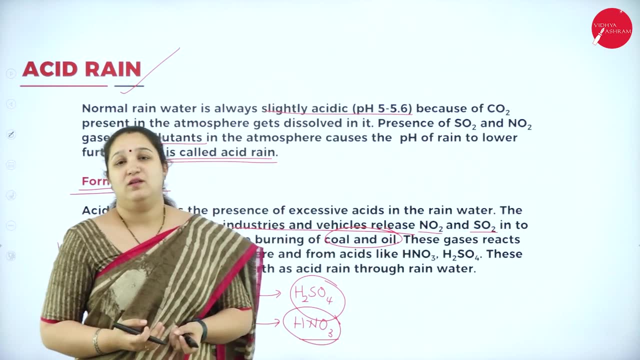 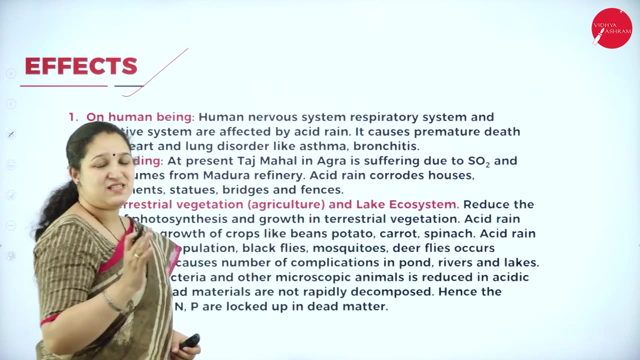 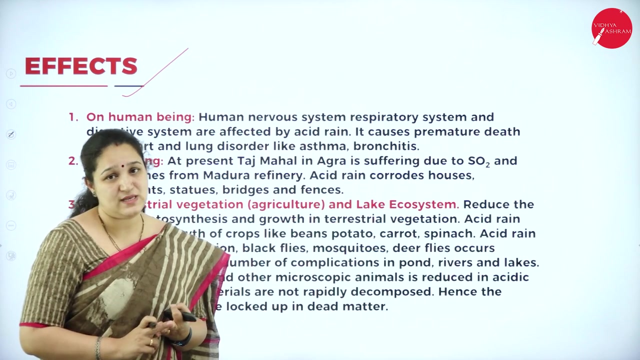 HNO3. so this is how we are going to get, or acid is formed, due to which, you know, the rain water which comes down will have pH less than 5.. Next is effects of acid rain on humans. acid rain has lot of effect on the respiratory system, nervous system, as well as the digestive. 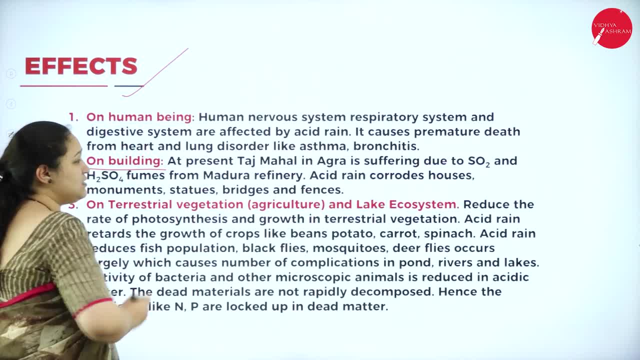 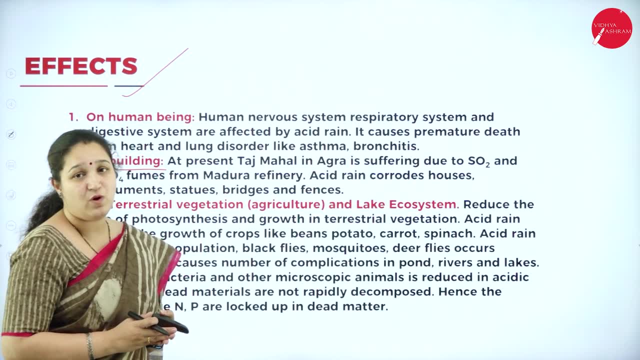 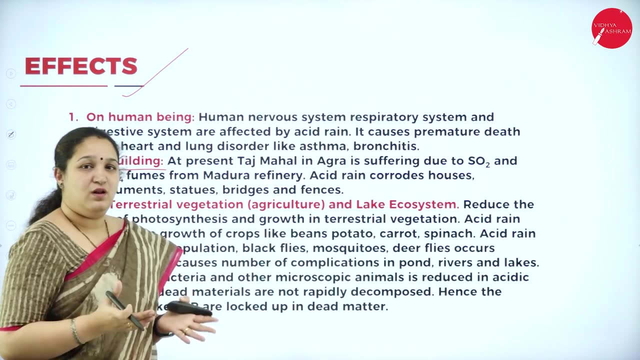 system and if you see on buildings, for example, Taj Mahal is getting affected with the sulfur dioxide gas as well as the sulfuric acid which is formed due to the Mathura refineries which is there very close to Agra, and the marble is getting faded off or you can tell it's getting. 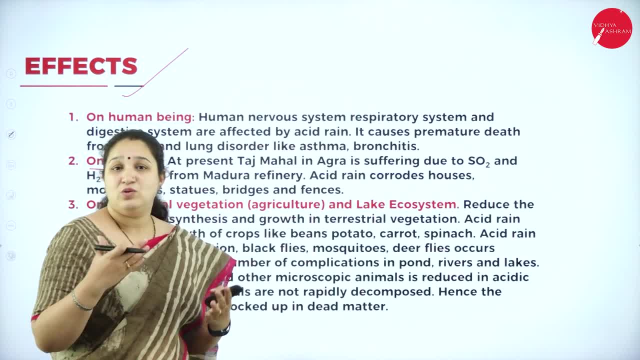 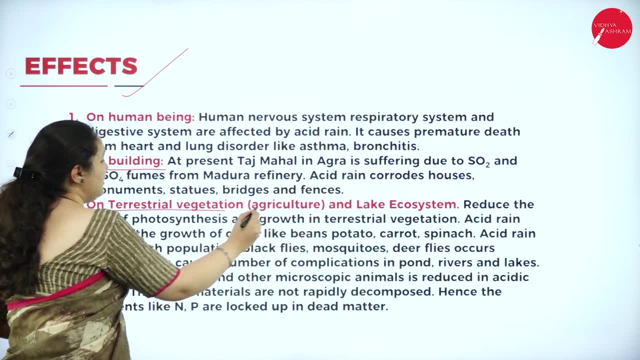 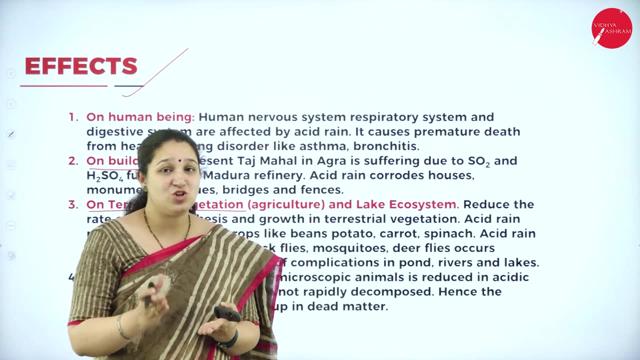 corroded. so the monuments, the statues which are there, you know, the buildings can get corroded because of the acidity of the rain and also on terrestrial and vegetation and in the lake ecosystem. if you see, the vegetation is getting spoiled because the soil pH is increasing. also, photosynthesis process can be slowed down because of the acidity. 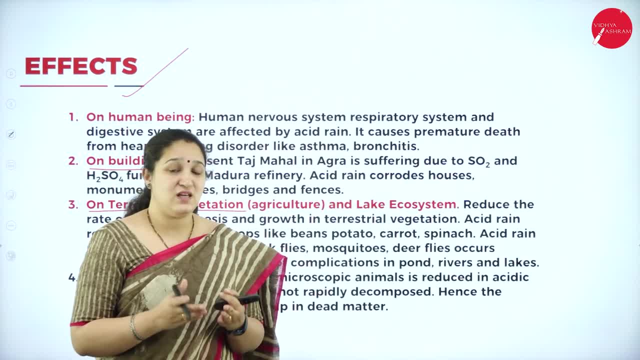 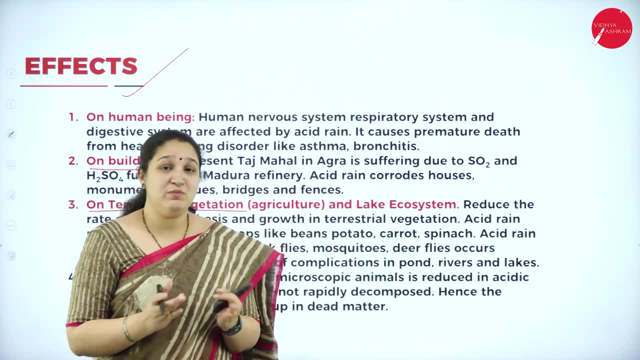 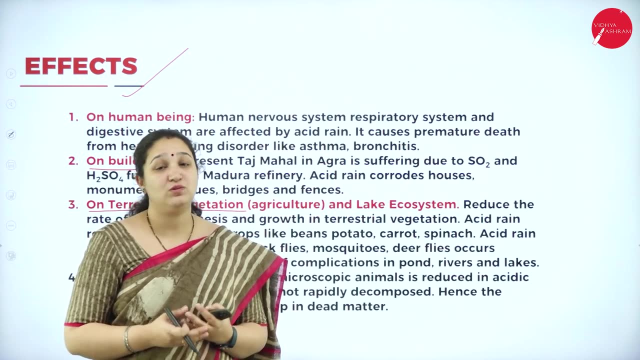 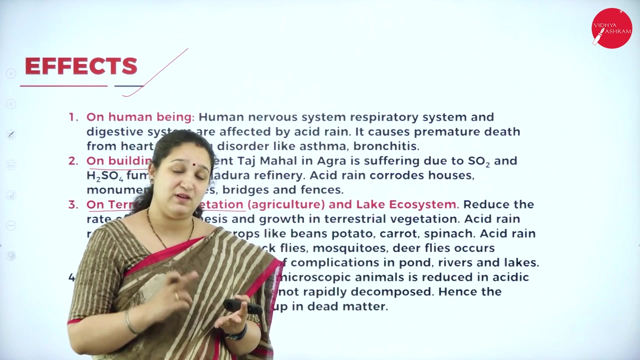 of water, and when these water, which is acidic, goes into the lake or river or pond ecosystem, they will, you know, diminish the growth of fishes and all the other microorganism growth or any aquatic animal growth can be, you know, largely affected and thus, you know, the lake ecosystem is affected, even the 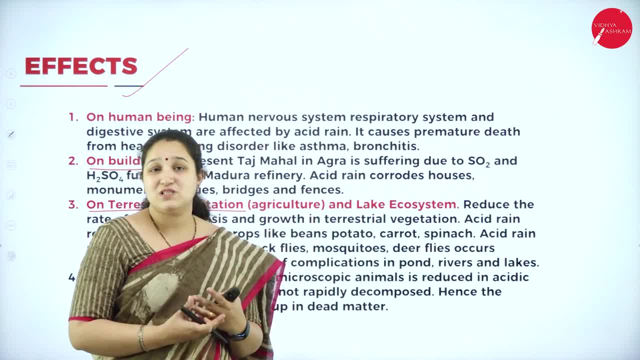 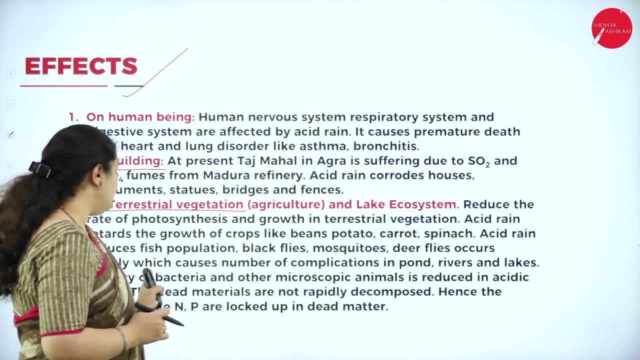 vegetation crop. what you yield is less. the photosynthesis process is becoming very, very less and thus affecting the vegetation as well as the ecosystem, and also bacteria and microorganisms are also affected because the acidity of the water and the sulfuric acid which is formed due to the 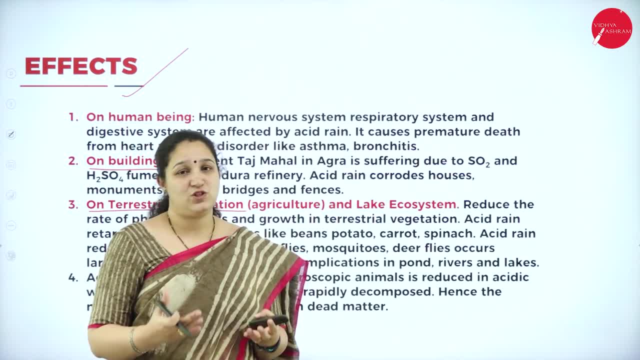 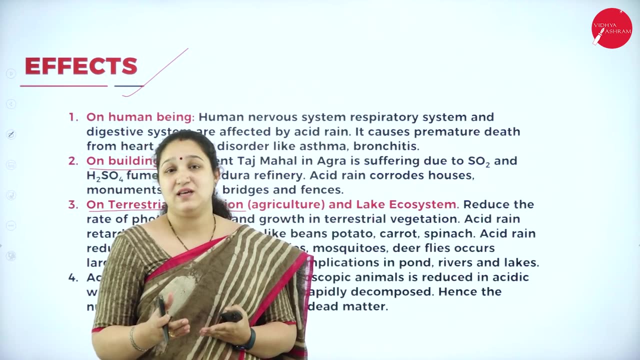 acidity is more, then only there is a certain type of bacteria which can work on it. some of the bacteria or the microorganisms cannot survive with the change in pH okay and the dead and organic matter cannot be decomposed very easily and the nitrogen, phosphorus etc. gets locked up in the dead matter. 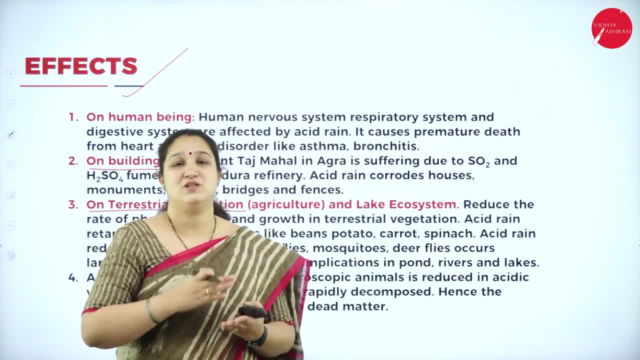 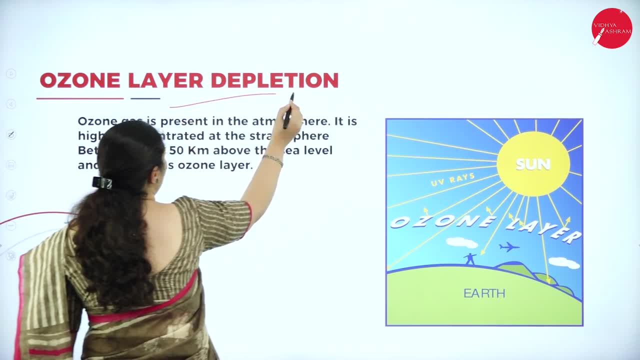 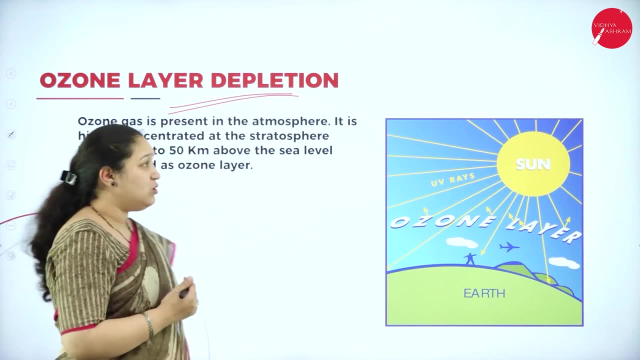 it is not going into the soil. the cycle of decomposition is again affected due to acid rain. next, if you see about ozone layer depletion. So what is ozone layer? okay, How is it getting depleted? ozone layer has got O3 and this layer is present. 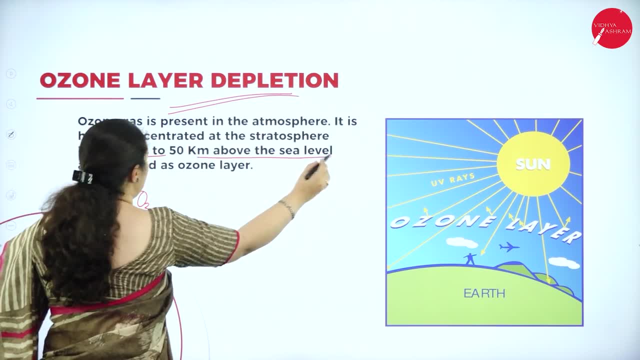 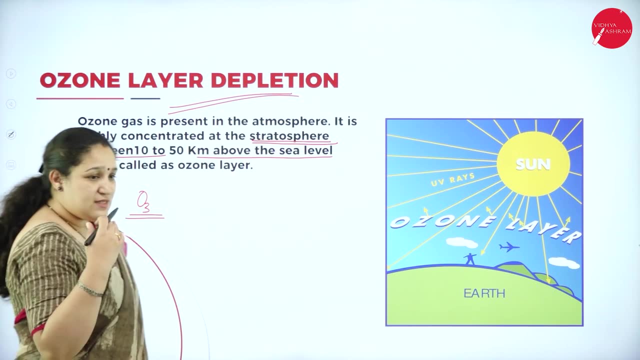 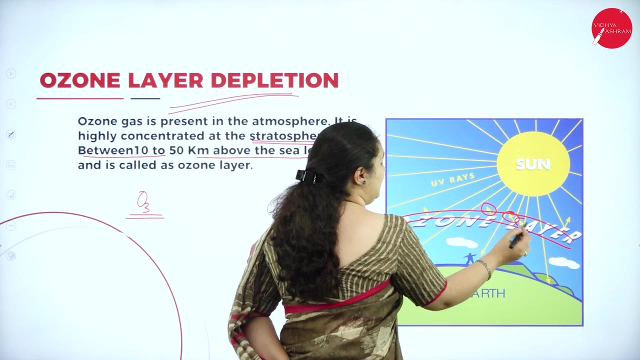 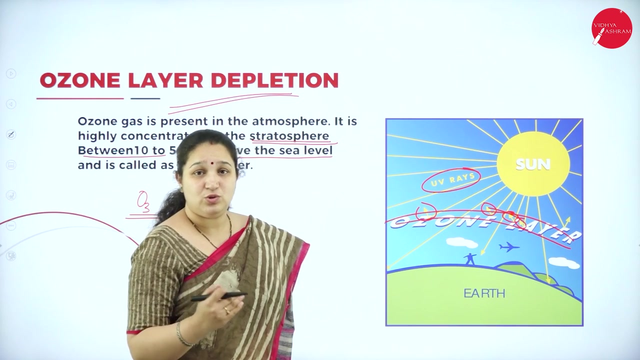 okay, in between 10 to 50 kilometers above the sea level at stratosphere, ok, in the atmosphere. so what is the function of ozone layer? ozone layer, which is present, okay. It will not allow total31 Atmospheric the UV rays from the Sun to enter the earth. okay, and due to this, there is lot. 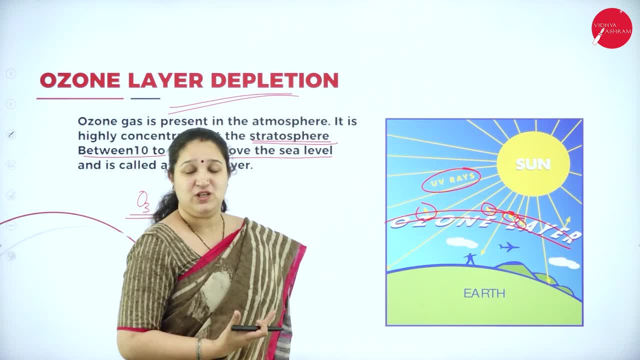 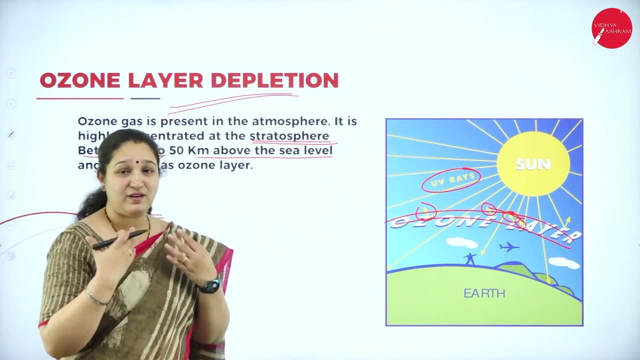 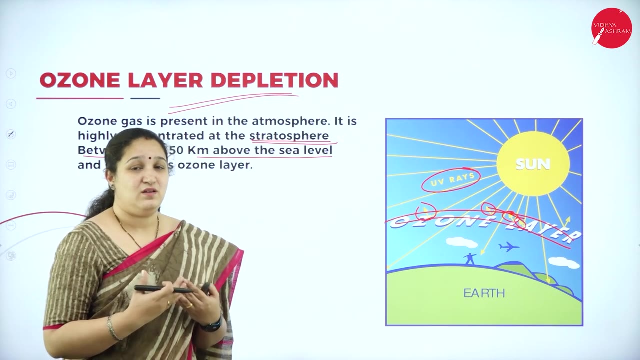 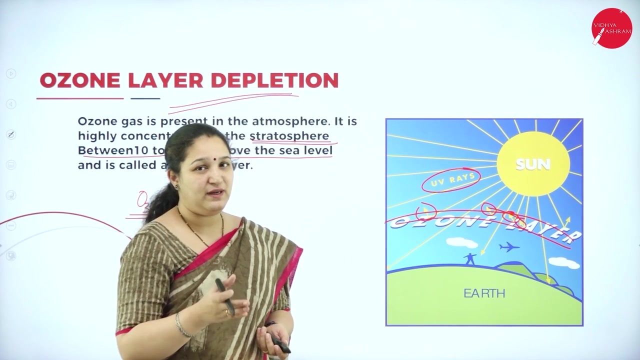 of you know uses for us especially is UV rays has got very bad effect on human health, like skin cancer or you know, it can affect our eyes, our skin, it can affect the plants, many, many things. okay, so all of this can be avoided due to the presence of ozone layer, and now the ozone layer is getting depleted. so again, 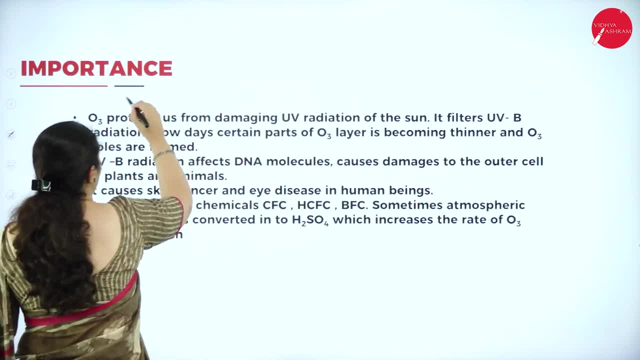 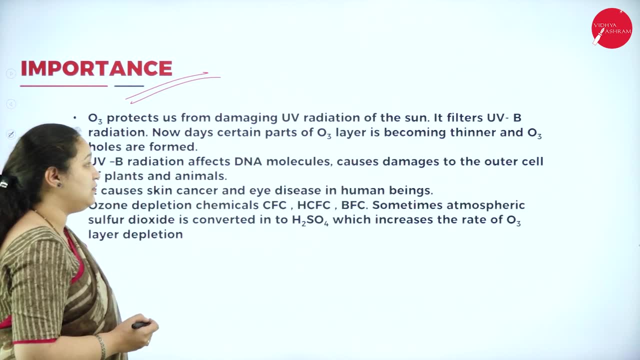 we are in problem, okay, so what is the importance of ozone layer? if you see, ozone protects us from damaging UV radiations from the Sun. it filters UVB radiations. nowadays, certain parts of ozone layer is becoming thinner and ozone holes are formed. UVB radiation affects the DNA molecules, causes damage. 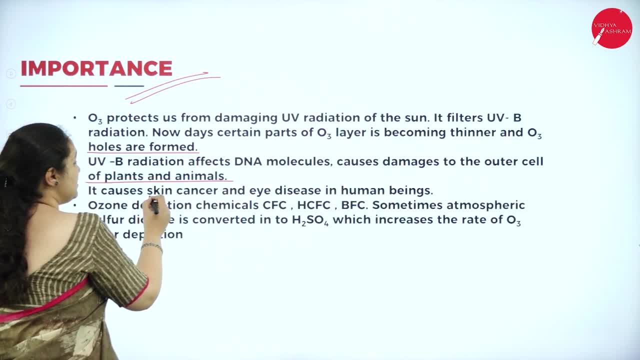 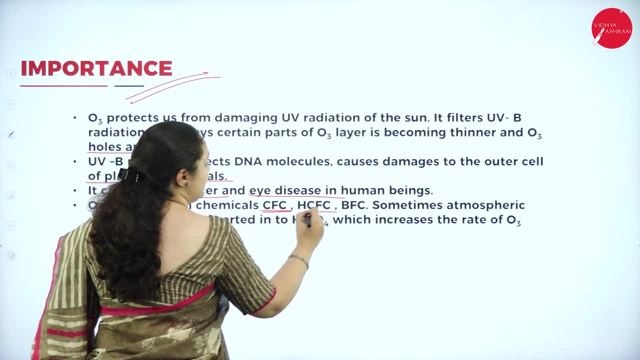 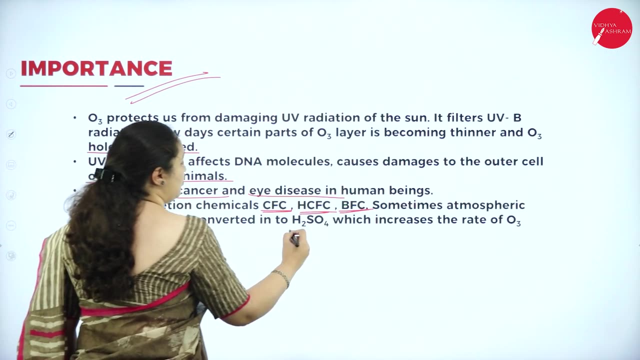 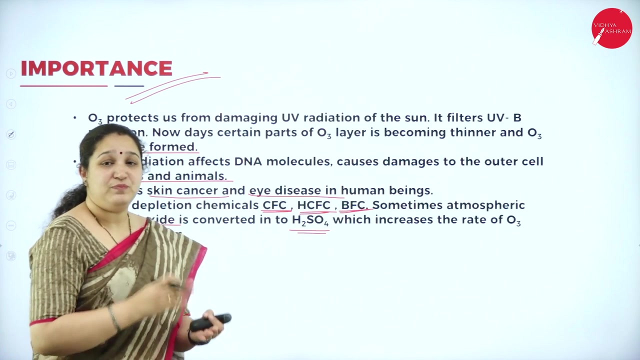 to the outer of the plants and animals. it causes skin cancer, eye diseases in human beings and ozone depletion. chemicals like cfc, hcfc, bfc. sometimes, you know, atmospheric sulfur dioxide gets converted into h2so4, which increases the rate of ozone layer depletion as well. okay, so you can see the main. 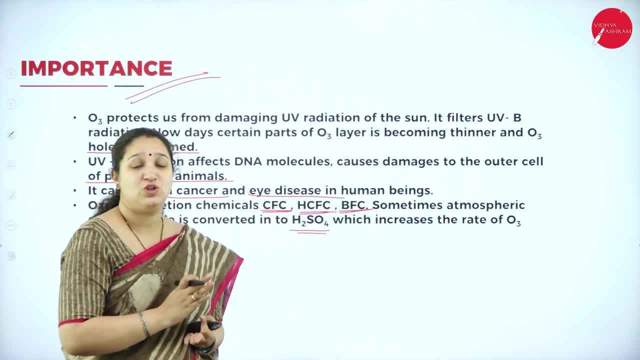 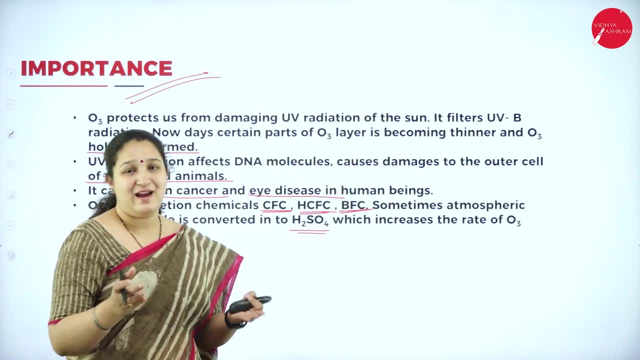 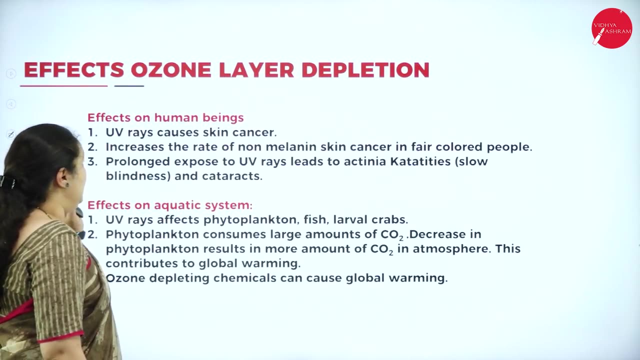 reason for ozone layer depletion is cfc's chlorofluorocarbons- okay, so if this content reduces the ozone layer can be protected and we can save ourselves from so many diseases which can be caused due to the uv radiation. okay, and also the effects of ozone layer. we'll study it.